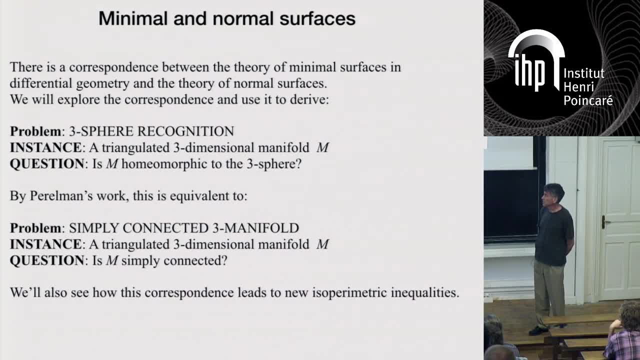 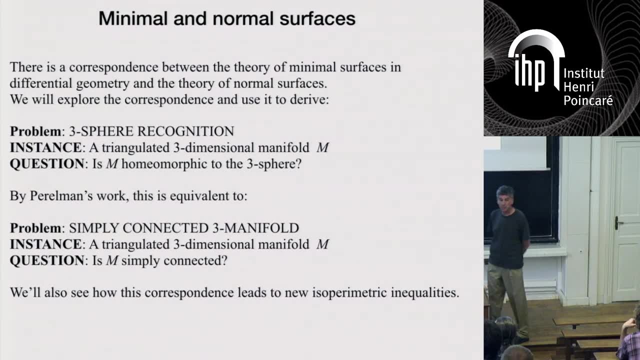 It's equivalent to asking whether the simplicial complex is simply connected, as we now know from Perlman's work. Now, one of the reasons people were interested in the problem was that it was a problem of the three-dimensional manifolds. One of the reasons this problem was to try to look for a counterexample to the point. 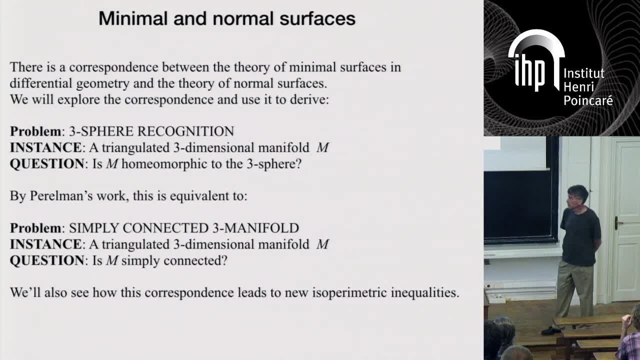 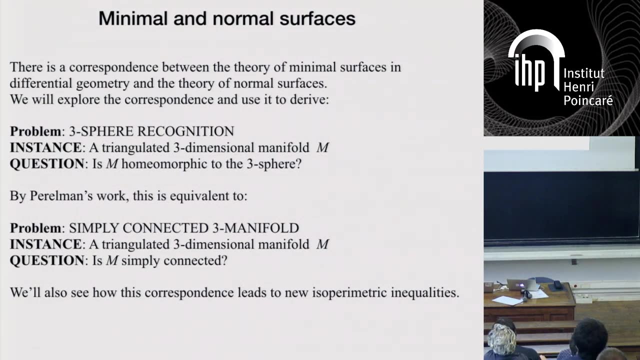 correct conjecture. In fact it wasn't even clear whether the point correct conjecture was decidable at that time, which now we know that it is. But remember, we still don't know whether the four-dimensional smooth point correct conjecture is decidable, So it's not. 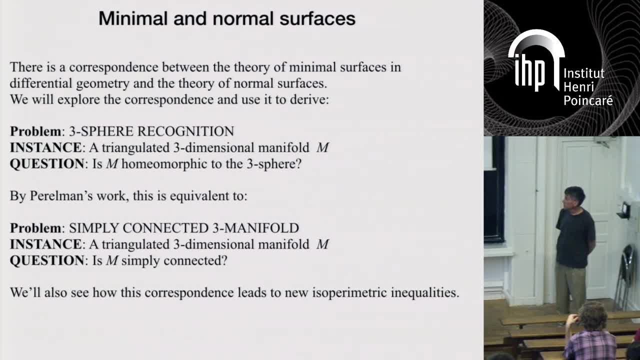 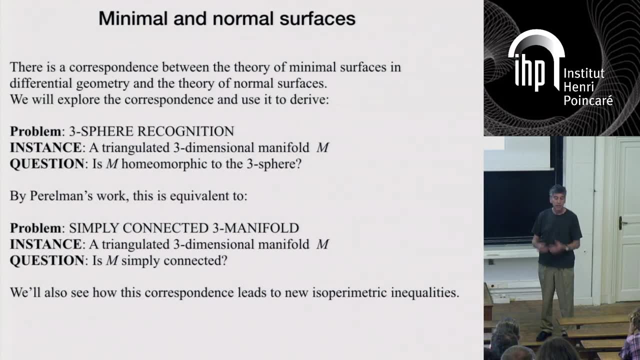 completely ridiculous to think that it might not be. Another place where the three-dimensional recognition problem comes up is in trying to determine whether a four-dimensional simplicial complex is a manifold. So if you have a collection of four-dimensional simplices and you want 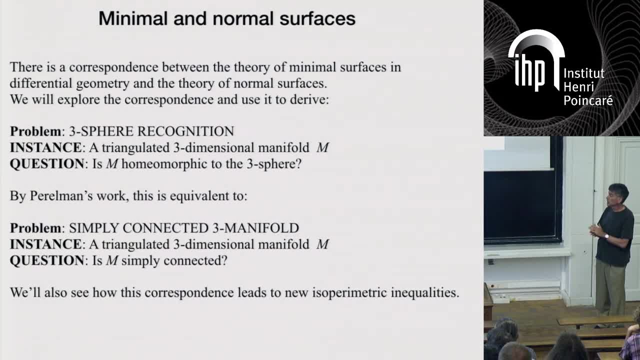 to see if they are glued together in such a way that they make a four-dimensional manifold. you have to check that. the link of a vertex, all the three simplices that fit around the vertex, form a three-sphere. I think that's actually implemented now in Regina, So it's actually being used. 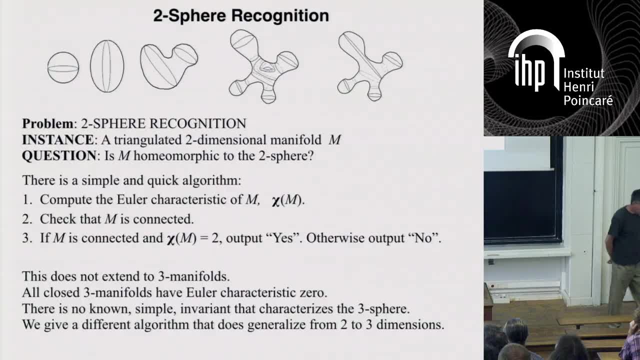 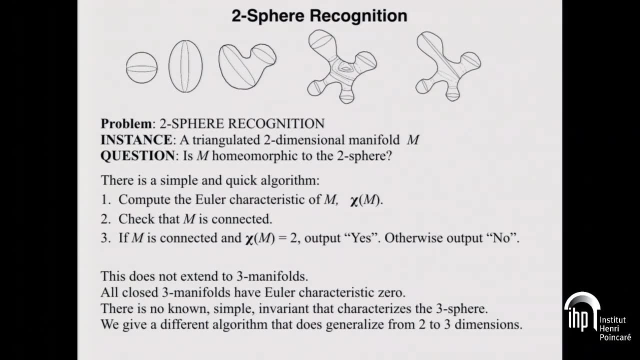 To understand the idea that led to the solution, let's step back and think about how we'd recognize a two-dimensional sphere. So if we have a two-dimensional complex, a union of triangles and cake societes, some of the edges identified in pairs, how can we tell if it's a two-sphere? 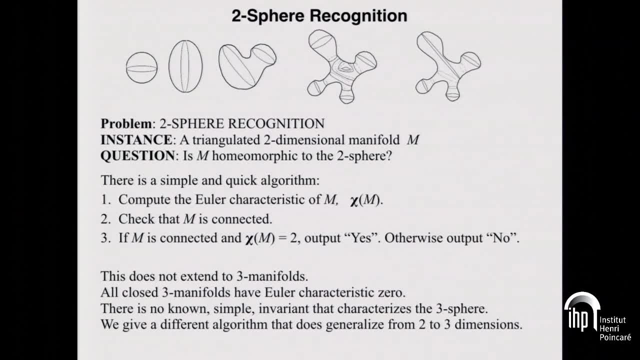 Well, the simple way is just to check the Euler Characteristic. If the surface is connected and its Euler Characteristic is two, our algorithm will just output yes and otherwise it will output no. So that's a simple algorithm, but unfortunately that doesn't generalize to a four-dimensional. system. I want you to find out how you can evaluate this transformation challenges. So step 1, step 2 is to apply the n-typeационale illusion which our commenter, just Vlad, hade made. when he Wish, I gave you a handbook of the mathematical solution by который we have to evaluate the algebra between: 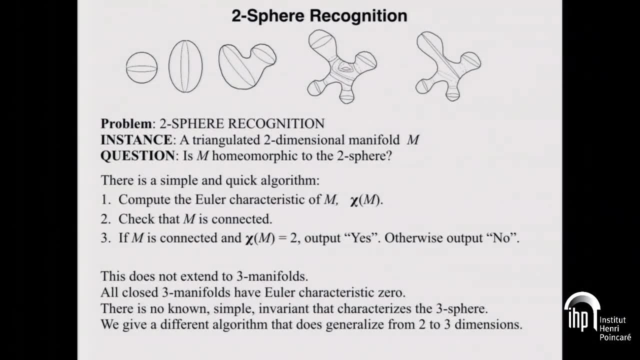 higher dimensions. There's no known invariant of three manifolds that distinguishes the sphere from other three manifolds and that is computable. So rather than doing this, we'll try and come up with a different type of algorithm, a harder algorithm for two-dimensional manifolds. 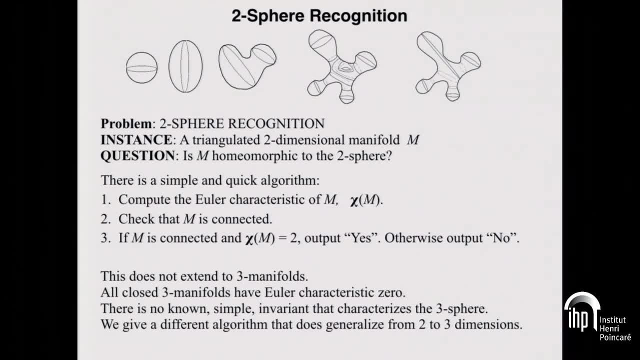 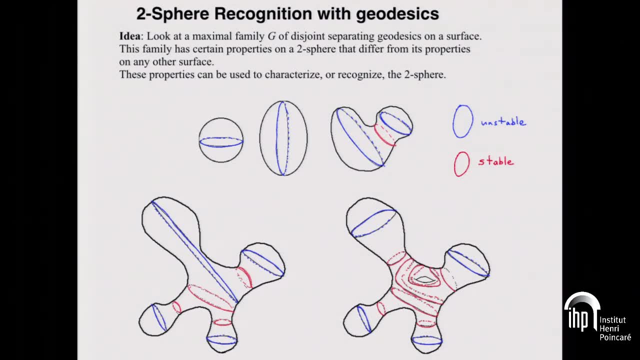 but this one will generalize to three dimensions. So what is the idea? The idea is to try and understand this system of geodesics on a two-dimensional manifold. So now we're leaving the world of simplicial complexes and entering the world of Riemannian manifolds. So these are smooth manifolds with Riemannian. 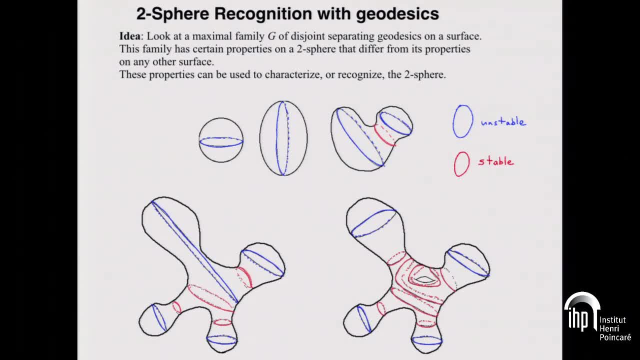 metrics And what I've drawn is just some examples of different surfaces and different types of manifolds. So what I've drawn is just some examples of different surfaces and the geodesics that lie on these surfaces. So the idea is we're going to 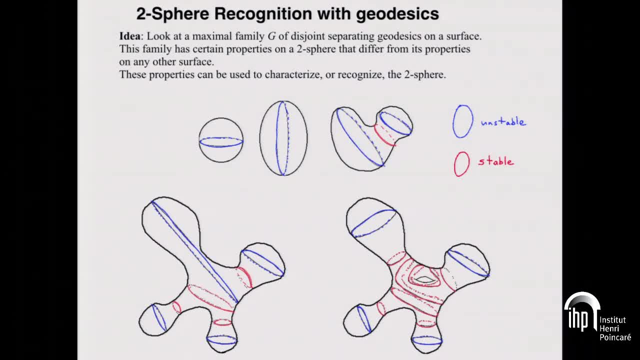 look at a maximal family of disjoint geodesics on a surface, So for example on a round sphere, that maximal family consists of a single equator. You have a lot of choices as how to pick that equator. There's many different. 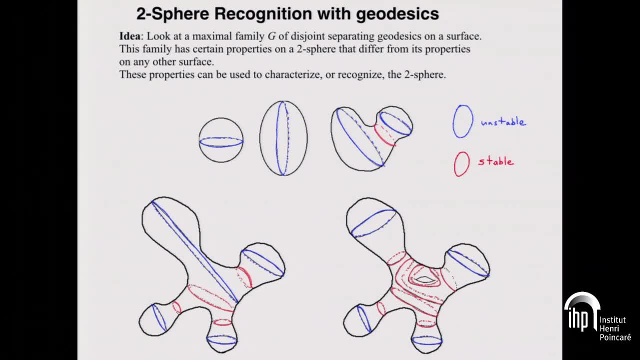 equators. but once you pick one, there isn't any other one that's disjoint from it. On an ellipsoid, you again would have one choice. You could choose one, but then there wouldn't be any others in the complement. But once you start getting, 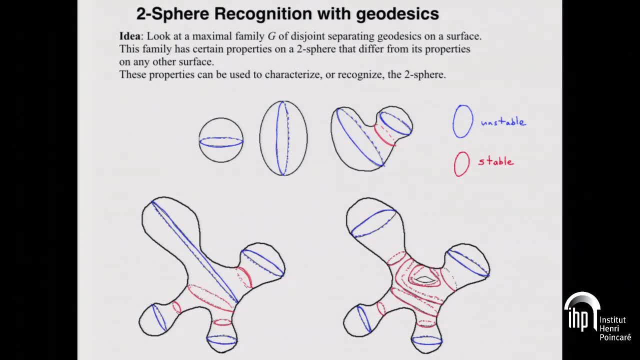 away from convex manifolds, convex surfaces. you'll see that there can be many disjoint geodesics, And these come in two flavors. There's the ones that I've labeled blue here and the ones that I've labeled red And the ones that I've labeled. 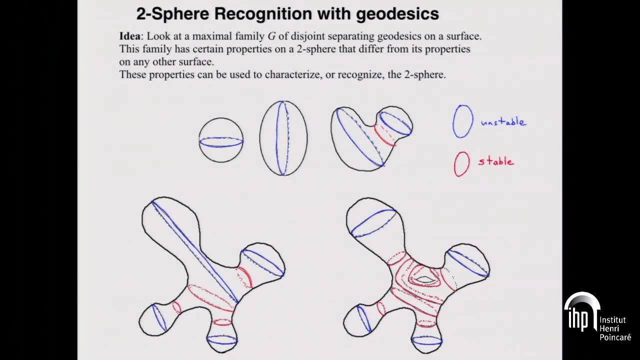 blue here, and the ones that I've labeled blue here, and the ones that I've labeled, that I've drawn in red, the ones I've drawn in blue. And the difference is, what's the difference between them? Well, if you think of these surfaces as being 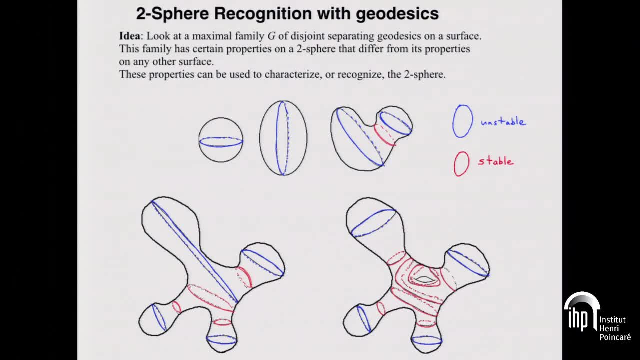 first of all cover them with butter, so everything's very slippery and can move around, and then take a rubber band and try and put it where these geodesics are. If you have one of these blue geodesics and you just touch it a little bit, it'll. 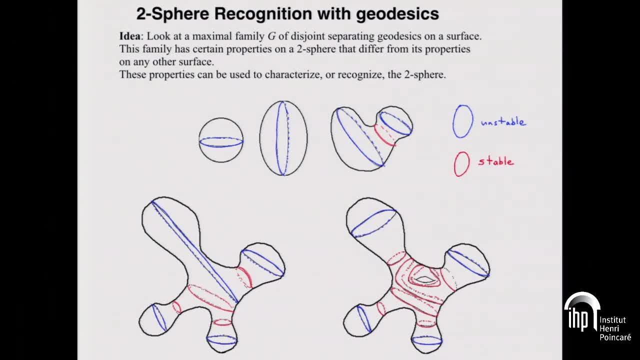 fly to one side or the other, But if you take one of these red geodesics, they're stable, They won't move. You could push them around and they'll just snap back to where they are. So, these red geodesics, 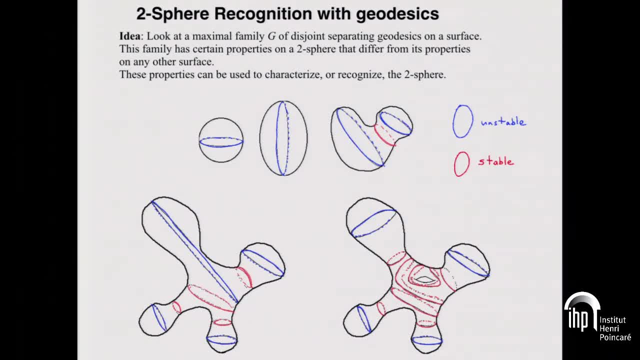 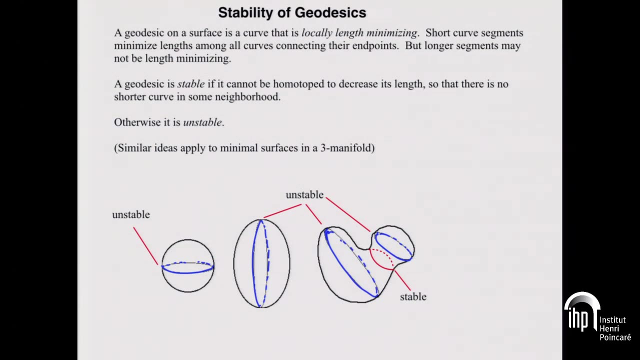 these stable geodesics are locally minimizing. they minimize length in some neighborhood, whereas the red ones, the blue ones don't. They're unstable. So let's look at this a little more. What's the definition of a geodesic? You can define it in various ways, but one. 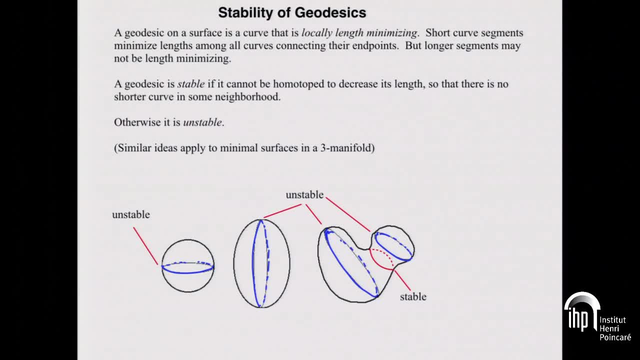 way is that if you take any two sufficiently nearby points, the geodesic gives you the shortest curve connecting those two points. So even on an equator, if you have two points that are close together, on the equator, the great circle gives you the shortest path between. 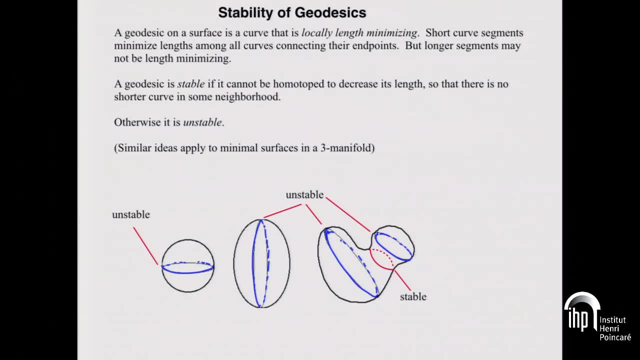 those two points. So that's always true for geodesics, But it's not true once the two points start getting far away along the geodesic. So we'll say that a geodesic is stable if there's some neighborhood of it in which 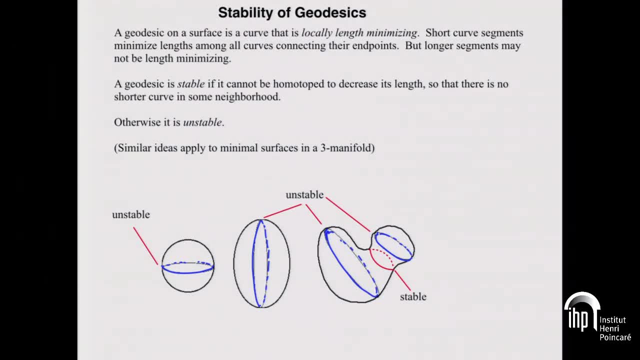 the entire geodesic, the entire curve is the shortest curve. So there's a little annulus surrounding that curve And the geodesic is stable And the area on the outer edge will be the shortest curve going around that annulus if it's stable And 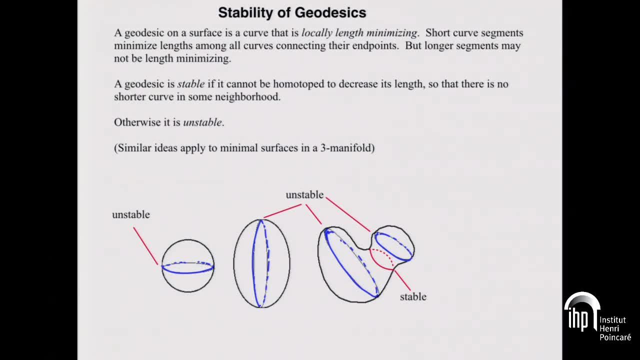 otherwise it's unstable. And there's similar ideas in higher dimensions. If you have a surface in a three-dimensional Riemannian manifold, you can look at its area and compare it to nearby surfaces. Minimal surfaces will be locally area minimizing. So if you take any point and a little, 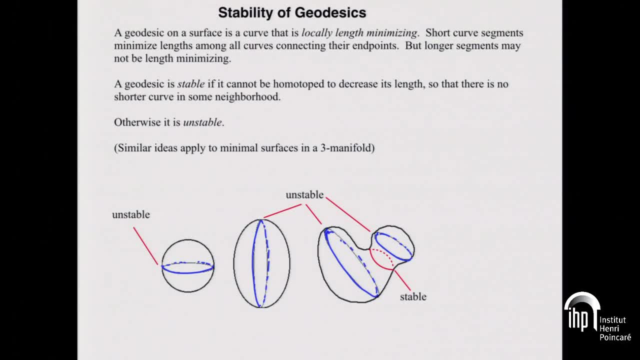 disk around that point in a minimal surface. that disk will be the smallest possible. it will have the smallest possible area among all surfaces with that boundary curve. But once you get bigger you can have unstable, minimal surfaces like the equator of a three-sphere which you can push off to. 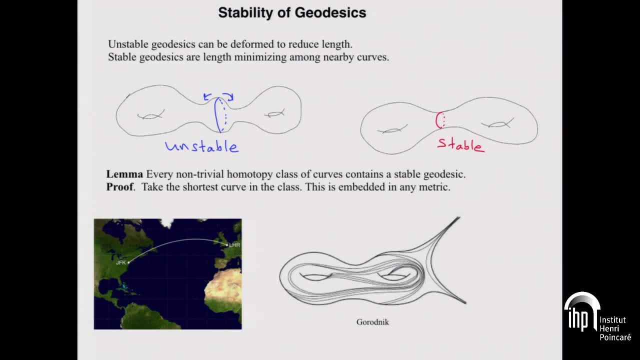 decrease area. So this is one example where I'm updating these everyday things. but with the changes of the expectations for future quadrevolution, There's some pictures of what these geodesics look like On the surface of the Earth. we see these when 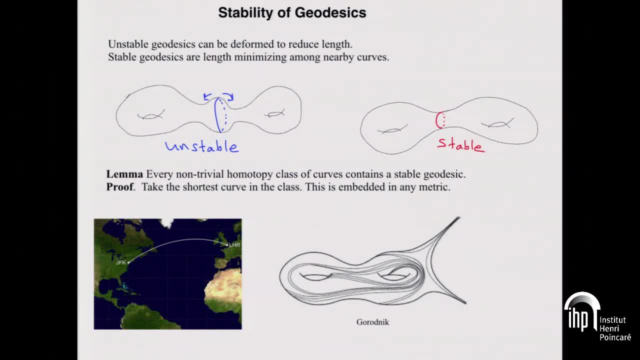 we fly on those airplane maps. the planes try to fly along geodesics connecting points, stable geodesics usually, And on surfaces. the basic lemma that we need to use is that subical is an ex pequenosma and there's a結齿 κ the핑,41 00 that, like in the neon shift�. 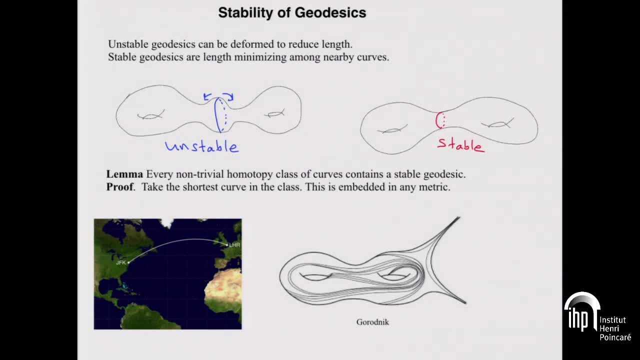 if you take any non-trivial homotopy class, any curve, that's not that you can't shrink to a point. you can always shrink it to a geodesic. It'll always have a geodesic in its homotopy. 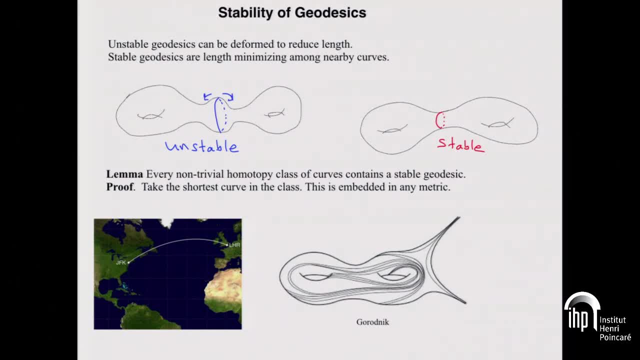 class and, in fact, if you take an embedded curve, the shortest geodesic will also be embedded. And this is true in any metric at all, not just in standard metrics like the hyperbolic metric on the surface, but if you take any metric at all. 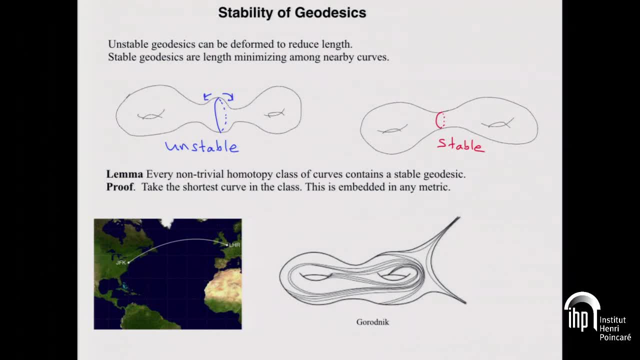 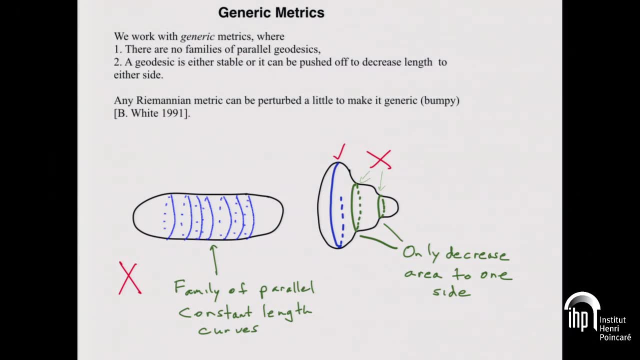 the shortest geodesics are always exist and they're always embedded. Now we're going to use for the. I want to actually state a theorem about these geodesics. so we have to make some assumption about the metric. We want to use a generic. 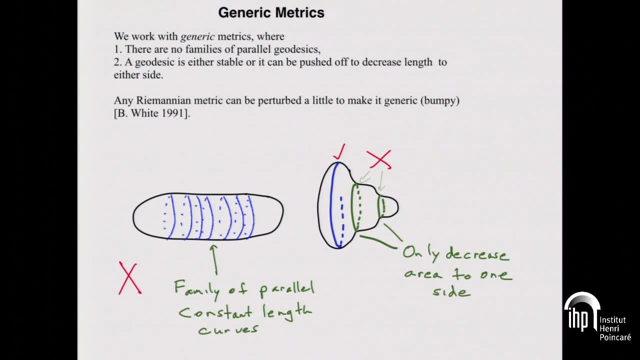 metric, and what that means is that you don't have some nasty behavior. For example, in a general smooth metric, you may have a cylinder piece inside a surface where you see a whole family of parallel geodesics. A flat cylinder has infinitely many. 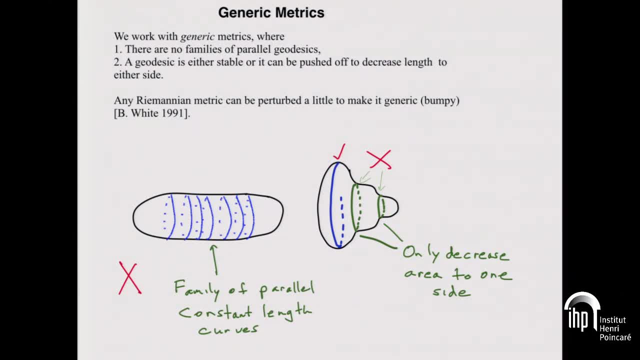 parallel flat geodesics. so we don't want to have to worry about those. You can't. you don't have to make this assumption, but it just makes the argument a lot harder if you have to deal with these cases. The other thing you don't. 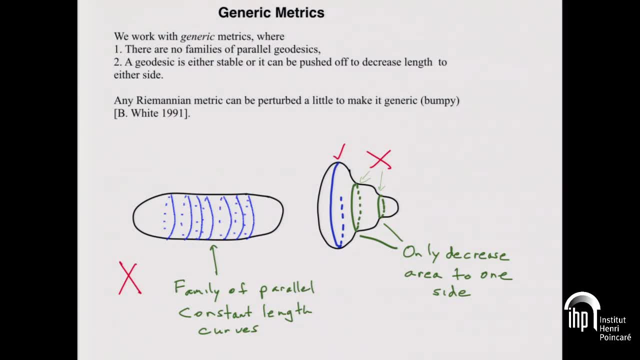 want is- you don't want these geodesics- that you can decrease area to one side, pushing them to one side, but not to the other side. See, if you have the equator of the Earth, you can decrease its length by pushing it to the south southern hemisphere. 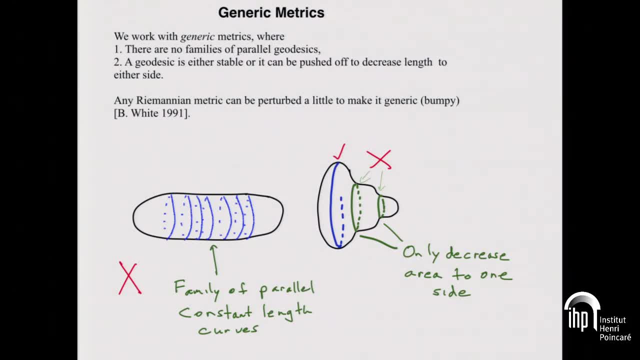 or the northern hemisphere, but you can't create these artificial metrics. They're very non-stable. though If you take a random perturbation of a metric, then you won't see these kinds of behavior, and that's actually a theorem in all dimensions. 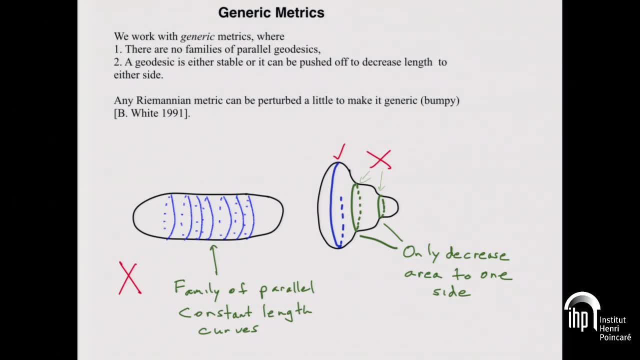 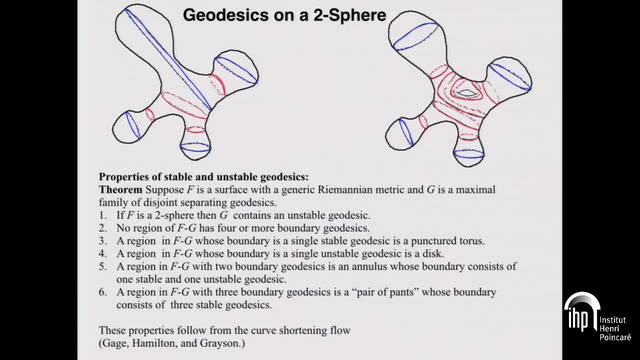 that was proven by Brian White in 1991.. It's called the bumpy metric. So what I'm going to do now is show you that if you take a generic metric on a two-sphere, then a maximal family of separating geodesics- excuse me, a general metric on any surface. 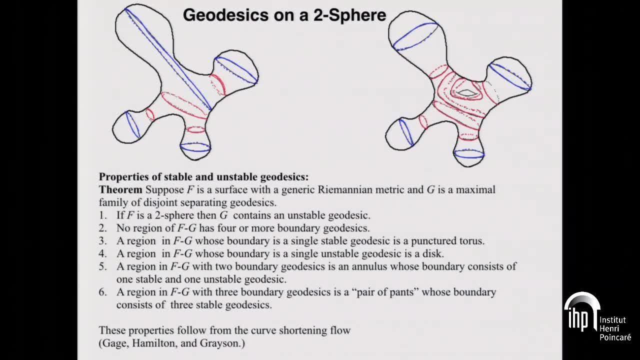 not necessarily a two-sphere. If you take any surface at all, the surface on the right is a torus and on the left is a two-sphere. If you take any metric at all on a surface, you'll find a two-sphere. If you take any metric at all on a surface, you'll find a. 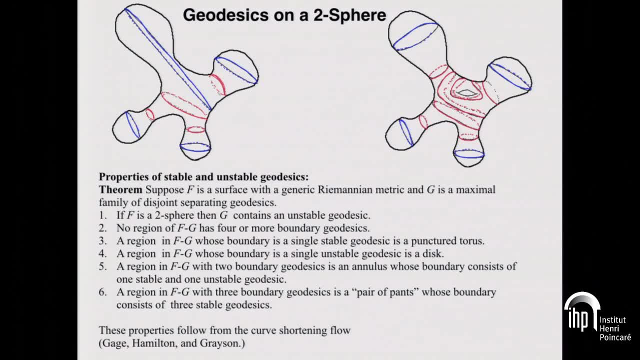 two-sphere, that a maximal family of separating two spheres has the following properties. First, if F is a two-sphere, then it always has an unstable geodesic. So what you see on the round sphere, that there is an equator, an unstable geodesic. 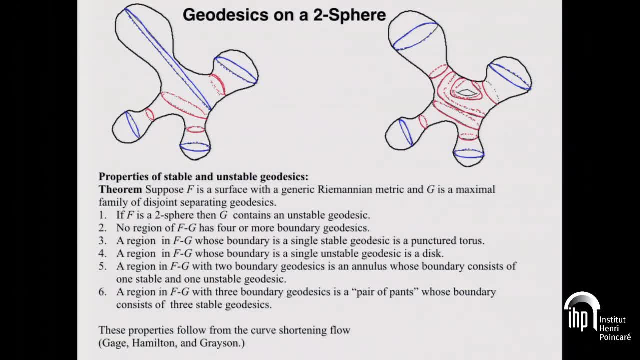 that holds for any metric at all on a two-sphere. This is a special case of an old theorem which has been extensively studied by different differential geometers. I'll show you the proof in a minute. It was first stated by Birkhoff in 1917.. There's been a whole series of variations on it- Listernick-Schnurman. 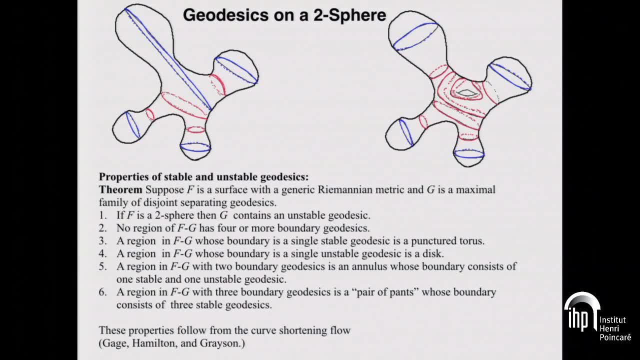 are two names associated with it, But there's various issues with the proof, associated with questions about whether the geodesic that these arguments produced was really simple or not, whether it was an embedded geodesic. But anyway, there's a very simple argument. 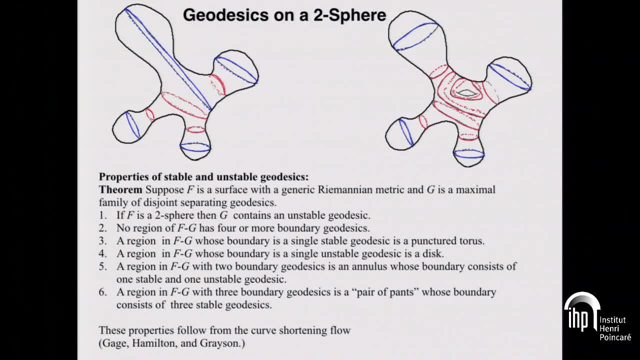 now based on the curvature flow theory that was developed by Gage, Hamilton and Grayson. So I'll show you that. Another property is that no region of the complement of this maximal family has four or more geodesic boundaries. So if you look at any of those regions, those surface regions bounded by that maximal family, 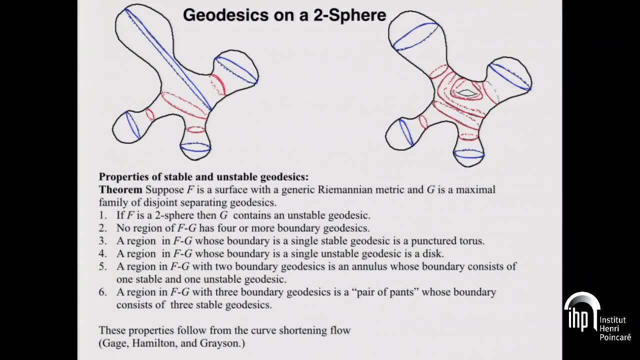 you'll never see a piece with four boundary components- And there's a few other similar results of a region whose boundary is a single stable geodesic has to be a punctuatoris. A region whose boundary is a single unstable geodesic has to be a disc. A region whose 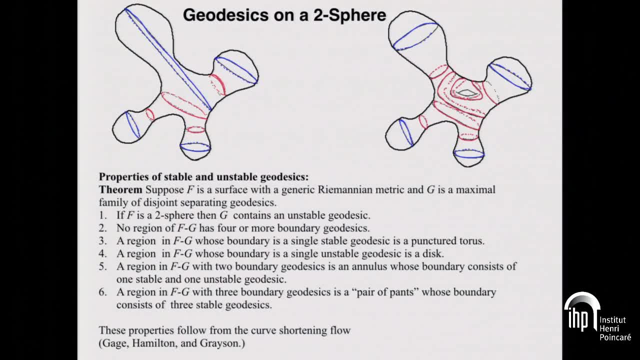 boundary has two geodesics has to be an annulus And it has to have one stable and one unstable geodesic. And the region which has three boundary geodesics has to be a pair of pants whose boundary has three geodesics. So this is pure differential geometry, but it's very simple. 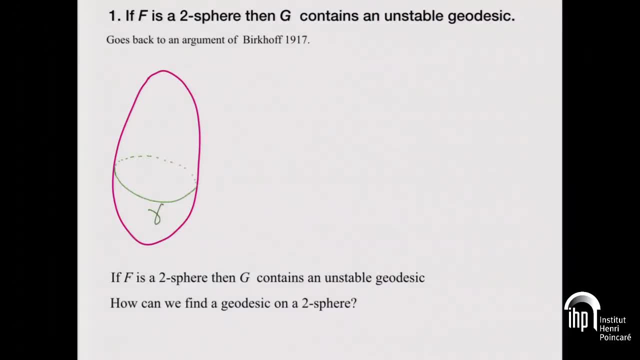 Let me show you the arguments, Sort of nice. So how do we see that any Riemannian metric on a two-sphere has to have a punctuatoris? Well, there's a very simple way to do that: have some unstable geodesic, some embedded unstable geodesic. 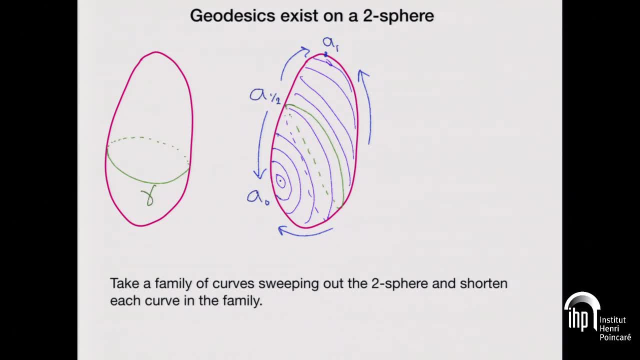 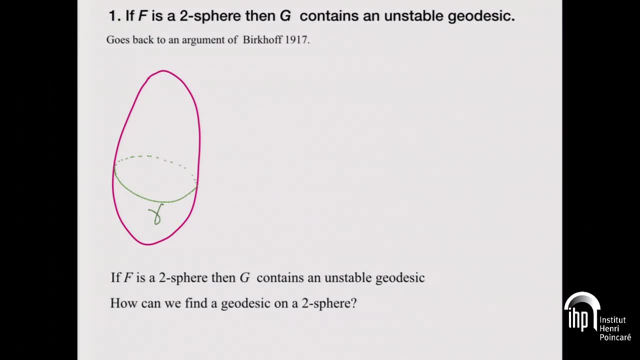 So let me show you this argument that goes back to Burckhoff. Excuse me, Yes question: Is there a way to remember this long list? Yeah, I'm going to go through them one at a time and then I'll put it back up for. 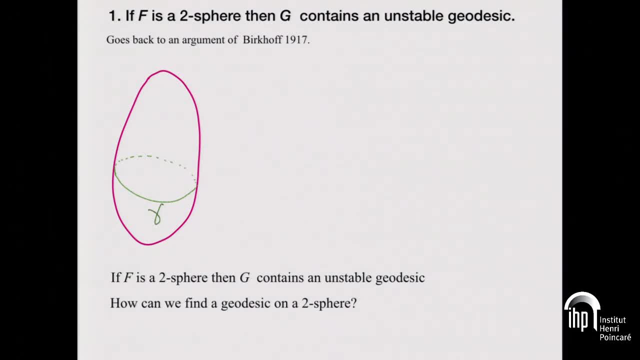 you so you can remember it. I mean, what's the organizing principle? Oh, what's the organizing principle? Well, there's either one, two, three or four boundary components and you just check the cases for each one, that's yeah or more, four or more, I should say. 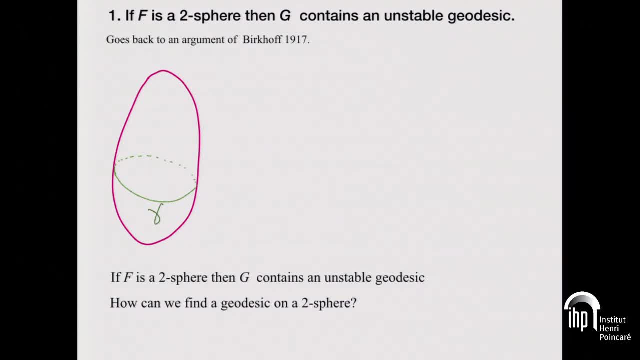 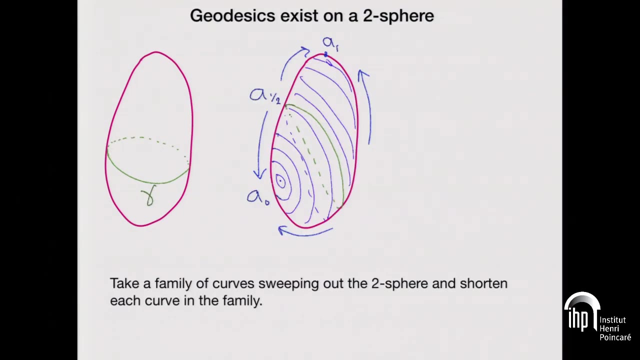 You just go systematically through each one. So let's say that there's a two sphere, This is a region with zero boundary components. How do we know that there always is an unstable geodesic Like the one that's drawn here? Well, what we do is we take a foliation, a family of curves that sweep out the two sphere. 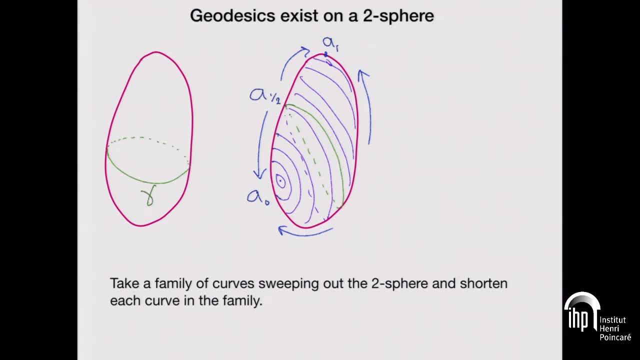 So all the you can think of all the lines of latitude on a sphere and the idea is to let them decrease in area all at the same time. Okay, Now, the original arguments didn't have that made. this, this is. I think this is. 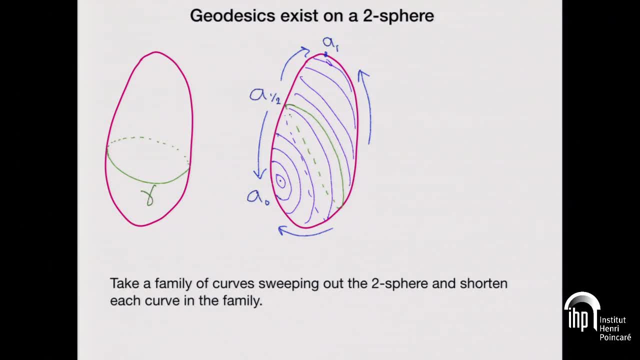 maybe Birkhoff, one of Birkhoff's most famous, one of the theorems Birkhoff is known to known for, at least in Wikipedia. it's one of two theorems that they list for him. He defined, he defined. he didn't have curve flows, so he made an argument like this, involving 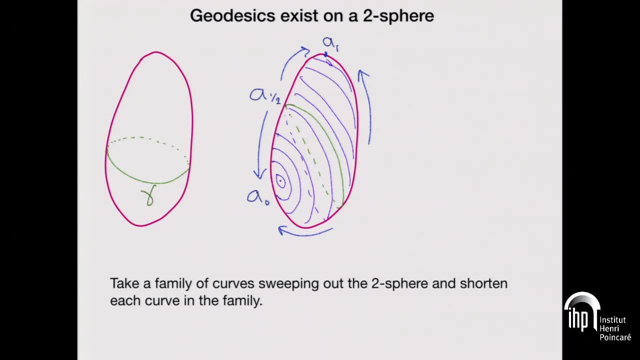 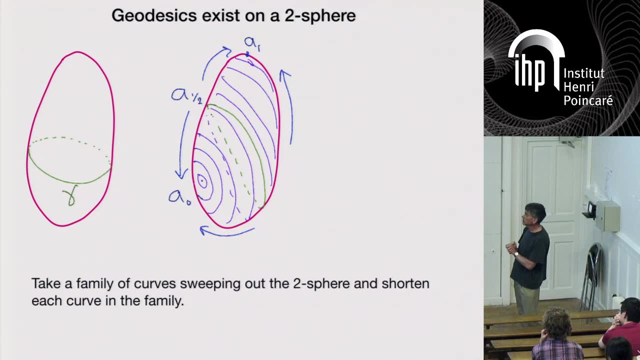 approximating these curves. He defined curves by polygons and flowing the vertices of a polygon and so on To shorten the, the polygon. But we today have this theory, due to Grayson and Gage Hamilton, that says that there's a canonical way to shrink a curve: by flowing by its curvature. 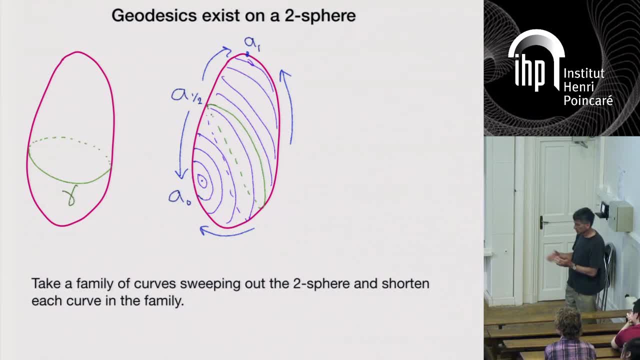 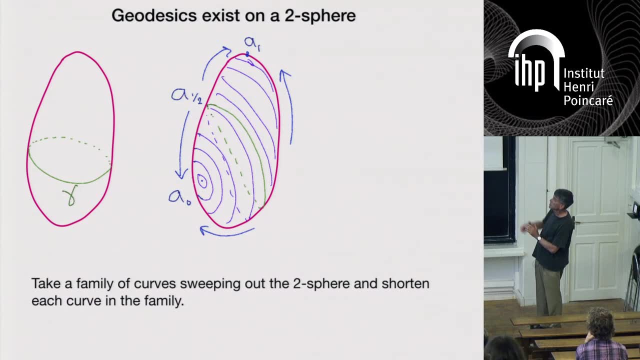 And if you apply that to this family, you'll get a continuous family of shrinking curves. Now the curve's near the point A0. You have this family, A sub A0.. Okay, A sub T is of curves, as T goes from 0 to 1.. 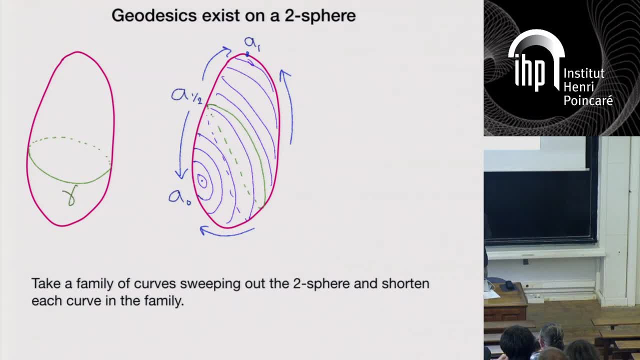 The curves near the point A0 will shrink towards A0. And the curves near the point A1 will shrink towards A1. And somewhere in the middle there'll be a curve that's. that's sort of stuck. It doesn't know which side to flow to. 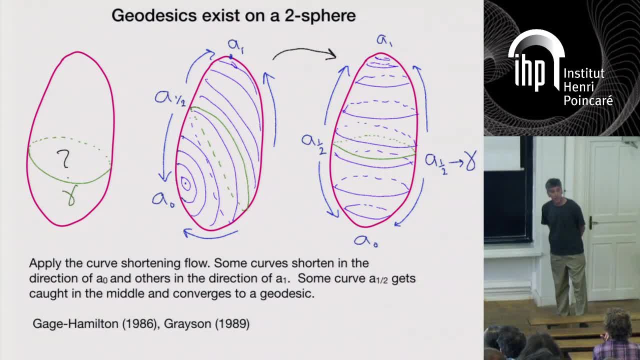 And if you think about what happens to that curve, you can show that it flows to a geodesic. Okay, Because this, the family- stays continuous. Okay, As as you flow and each curve gets shorter with time. So there's some limiting curve there which is a geodesic, and if you push it off to either 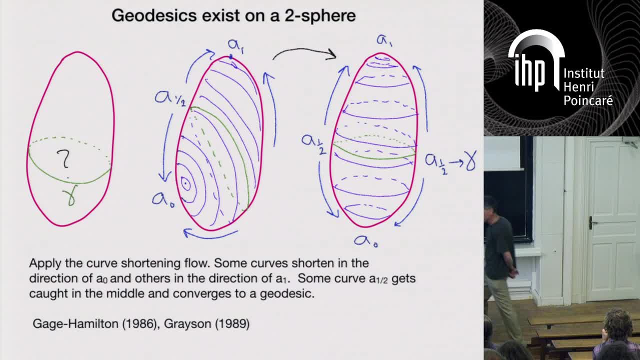 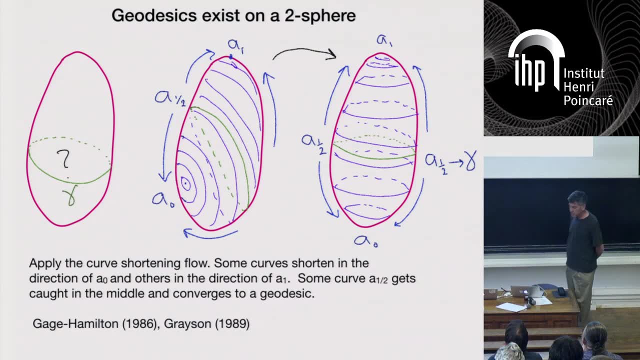 side you you'll get shorter curves. One of the interesting theorems is that in fact you can always find at least three such curves, And one of the nice theorems that Morse proved was that on an ellipsoid, if you take an ellipsoid, 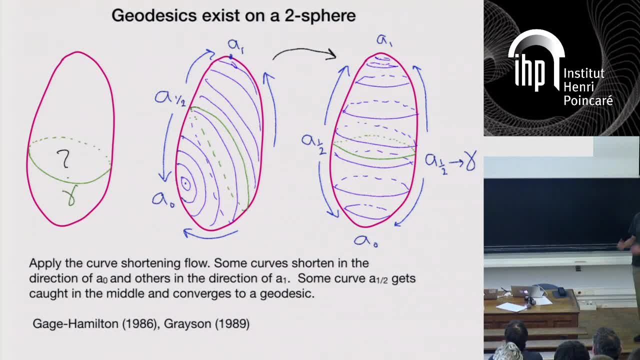 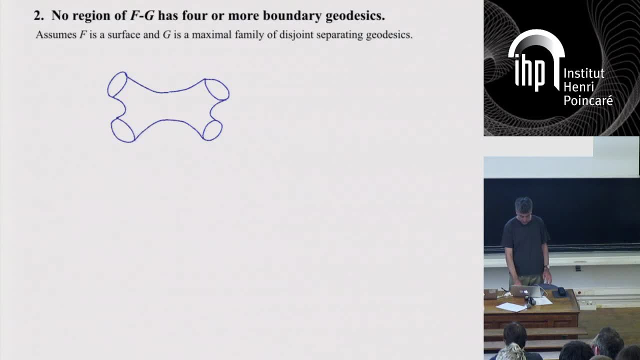 that's very close to a round sphere. there'll be exactly three. The three axes of the three symmetry planes will give you exactly all the simple geodesics on some ellipsoids. Okay, So let's look at four or more boundary points. 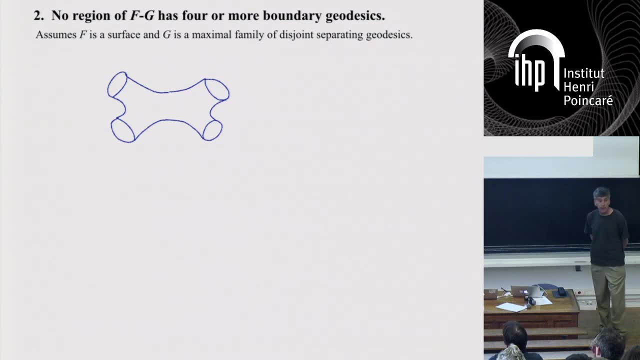 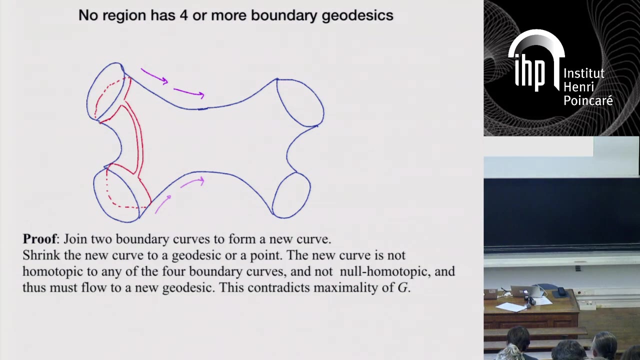 And show that these kinds of regions never appear in our maximal family. So you take any surface and take this maximal collection of separating geodesics, you'll never see a region with four boundary curves And the reason is: just take two of those curves and two of them together join them. 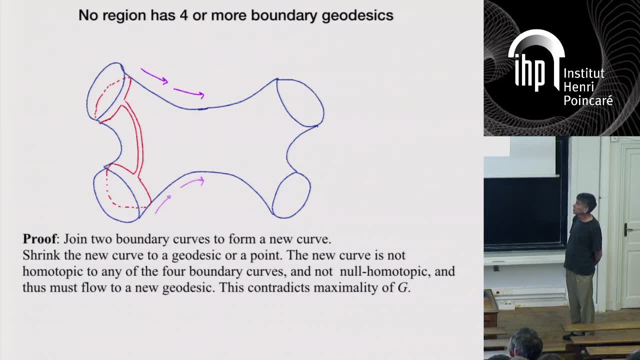 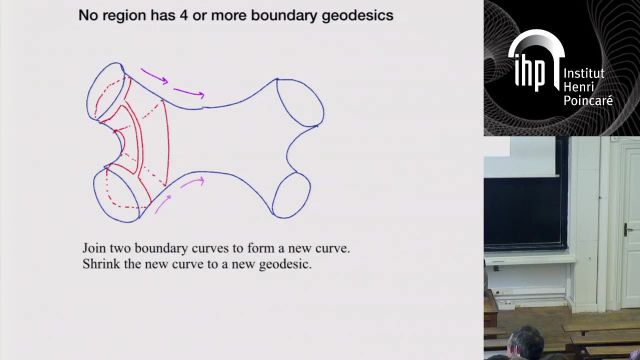 together by in this way and you get a new curve Right Which is not homotopic to any of the boundary curves. In fact it's homotopic to the curve in the middle that splits those boundary curves. But every homotopic class of curves has a geodesic 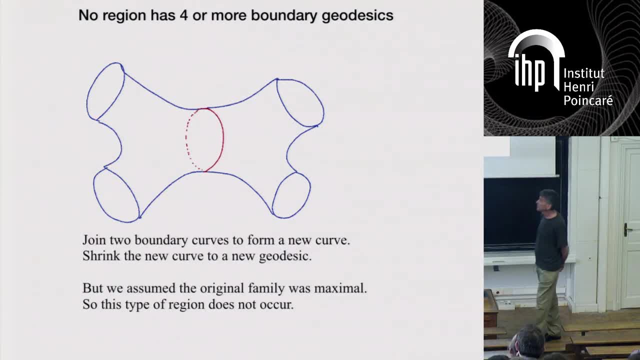 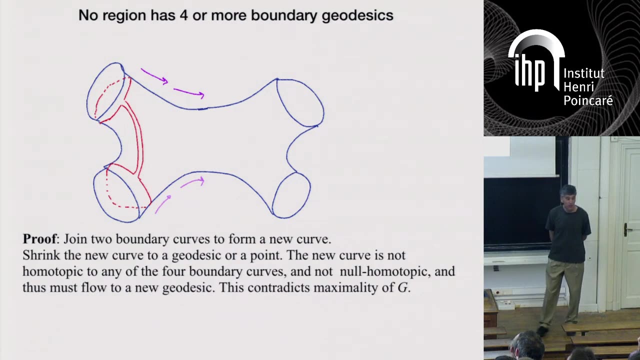 So there's a geodesic somewhere here in the middle that's homotopic to the sum of those two boundary curves on the left. You want to see that again? I see a couple of suspicious faces there. Yeah, See, So we took these two boundary curves and we formed a new homotopic class of curves, just. 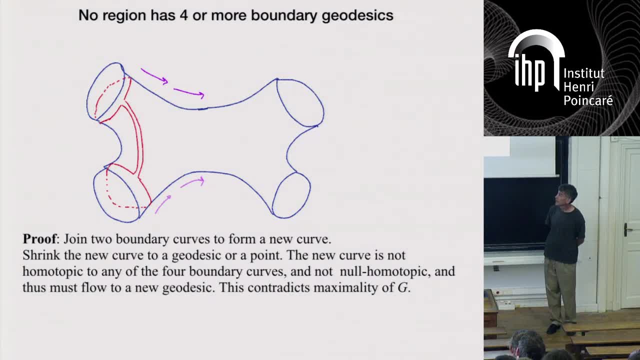 by joining them together like that right, And that's a curve which is simple and it's not homotopic to any of the four boundary curves. Well, so I said there was this basic theory that says that on a surface, you can represent. 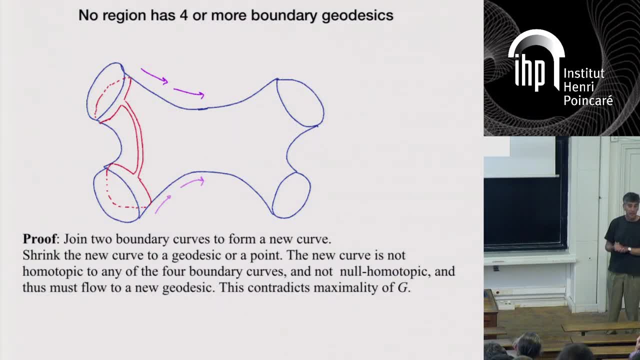 any homotopic class by a geodesic, So that curve has a representative by a geodesic. You might object to the fact that this is a surface with boundary, But as long as the boundary is geodesic, there's no problem in proving it for that case as well. 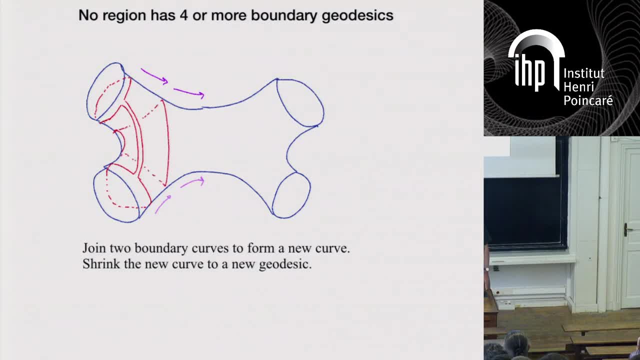 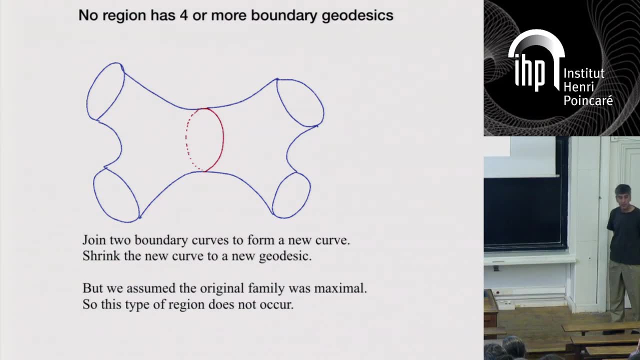 So the shortest curve, homotopic to this red curve, must give you something that is separating, because each of the original curves was separating, So this curve is separating as well. It wasn't in the original family, So the original family was not maximal and we see that this kind of region doesn't occur. 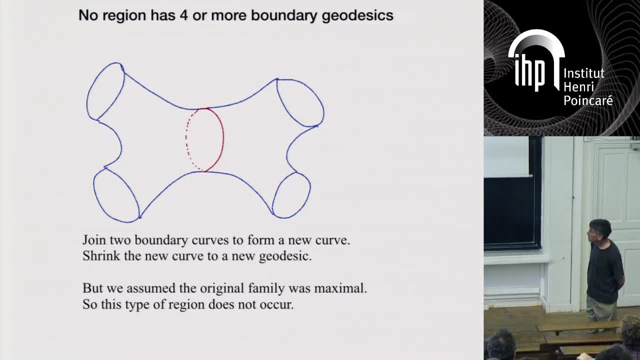 Yes, Can the red curve touch one of the boundary components Right? So topologically it could. but geodesics have the property that if they touch in a tangent then they're equal. They're determined by their tangent vector at one point. So it doesn't occur for geodesics. 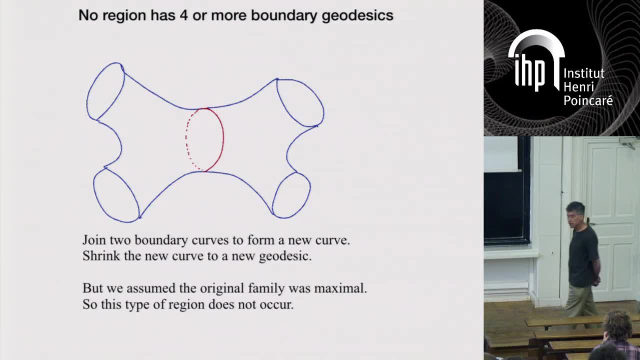 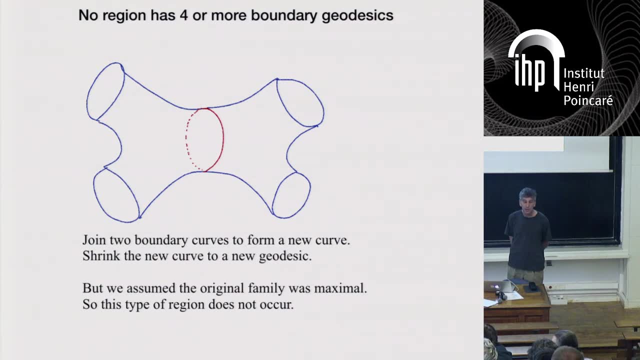 And the same is true for minimal surfaces. It's a… It's an important property that's used in this. Any other questions? Can you repeat the question? Oh sorry, The question was: is it possible for this red geodesic that's produced in this way? 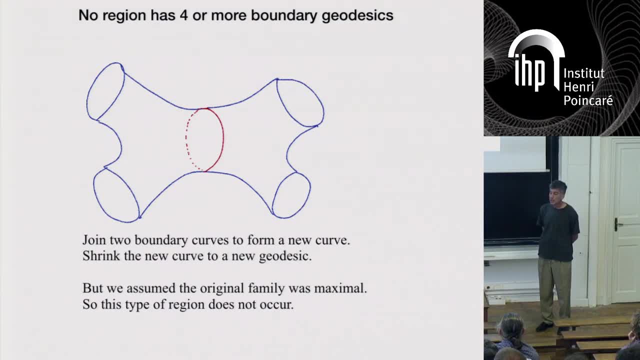 to touch one of the blue geodesics, And if… In fact, if they weren't… If the boundary components weren't geodesics, if they were arbitrary curves, then that could certainly happen. It could run along the boundary for a while. 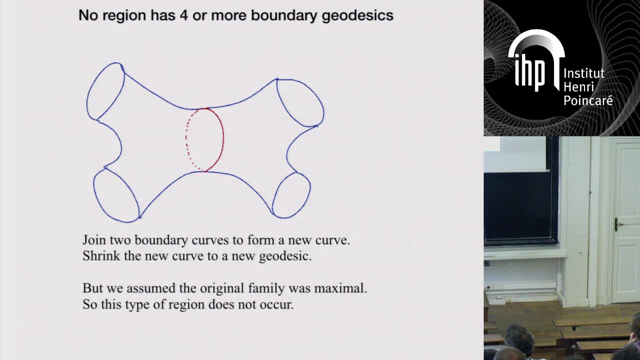 The shortest curve. But because they're geodesics and geodesics are determined by differential equation… First order, differential equations. you can't have two of them touching and tangent Any other questions? Yes, Is there an argument for why this is never contractible if it doesn't rely on like? 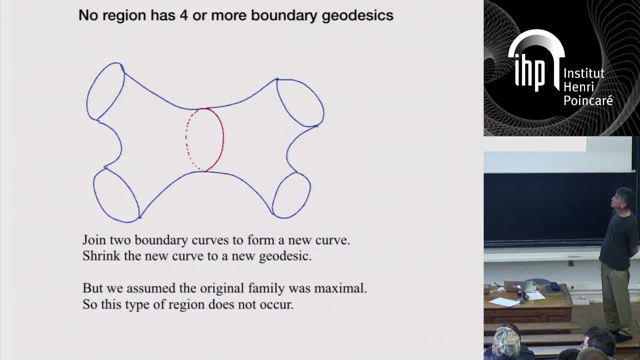 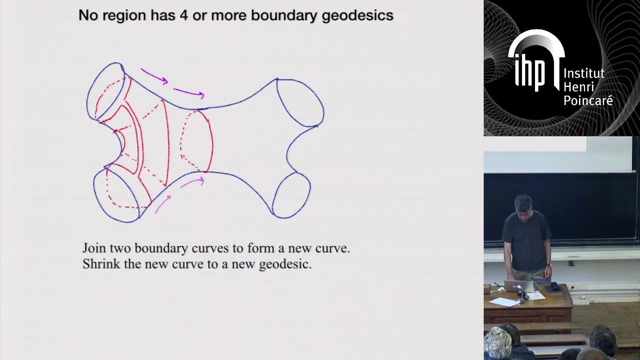 heavy, fundamental blue machinery Of why the union of those two isn't contractible. When you…. Yeah Well, you could say, for example, that…. So the question was: is there a simple argument how you see that this red curve that we constructed? 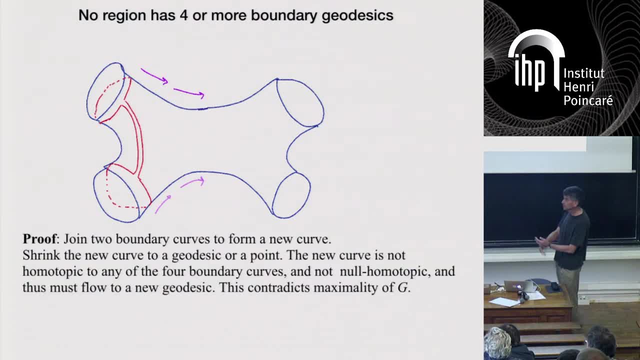 doesn't contract to a point And of course you could compute it in the fundamental group. but there was a question of whether there's an easier way. I think there is If you take the very top arc connecting the top left circle to the top right circle. 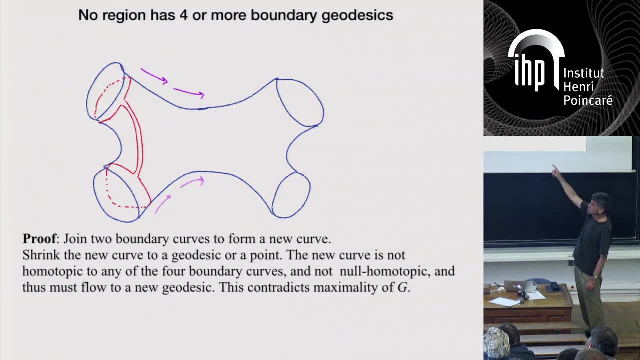 so the arc connecting those two boundary curves, that crosses the red curve once right And the contractible curve has to cross anything twice, So you can sort of use its separation properties. The fact that it separates two of the boundary components shows that it can't be contractible. 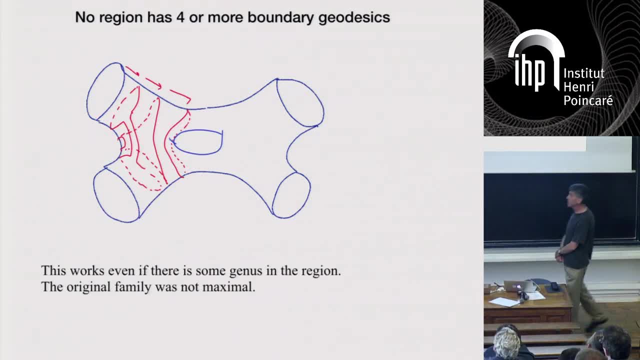 Okay, And I didn't cheat by drawing it like that. Even if I'd had some genus in there, the same argument would apply: You're getting a new homotopy class, and if you take the minimizer, you'll get a separating. 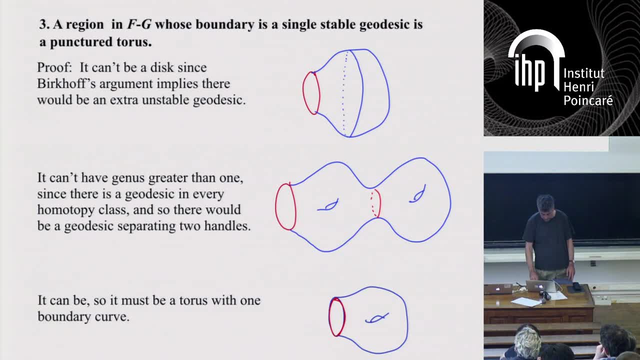 curve. that was not in your family, Okay, So next case: What about if there's a single boundary component? So there's going to be two cases: If it's stable or unstable. So we'll first look at a single boundary component which is stable, meaning that. so 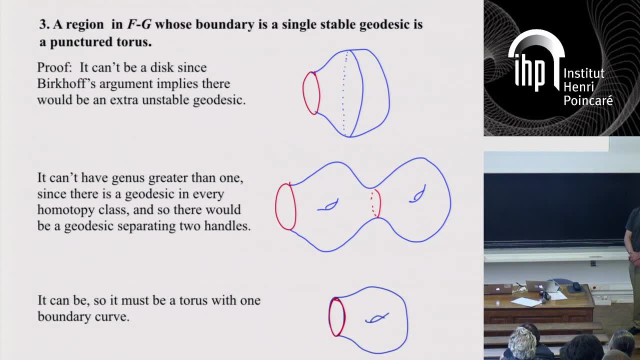 we look at that red curve and we assume that all nearby curves are longer. right, It's stable. So there aren't any nearby curves that are shorter. So that means when you push in you must be getting longer. Now we have two possibilities. 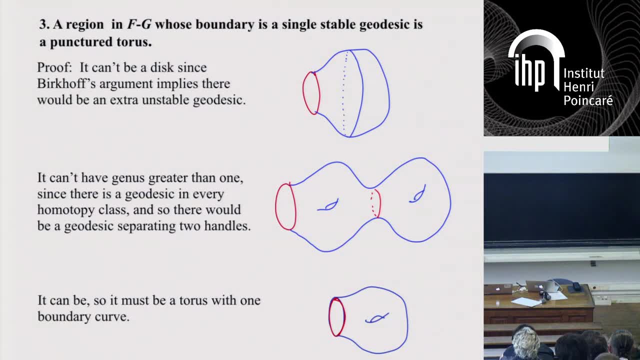 In the top possibility we see the case where that red curve is the boundary of a disc. Okay, And then the Birkhoff-Gage-Hamilton argument applies again. We get longer and then shorter So we can find we can run curve flow and we can we get stuck on some blue curve in. 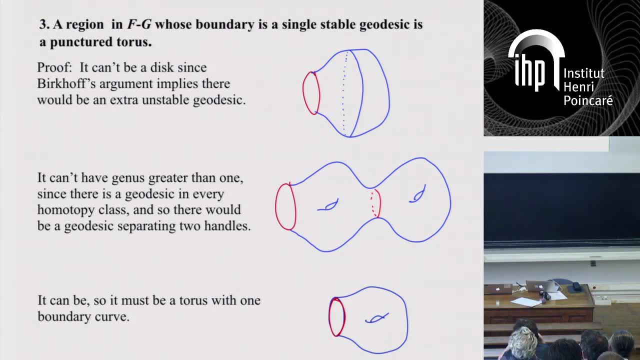 the middle, which is a geodesic. If it's not a disc, then there's. it's got some topologies, So it could have two. it could have more genus more than one. It could bound the surface with genus more than one. 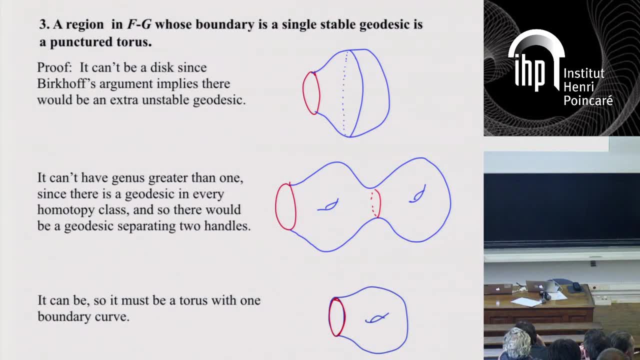 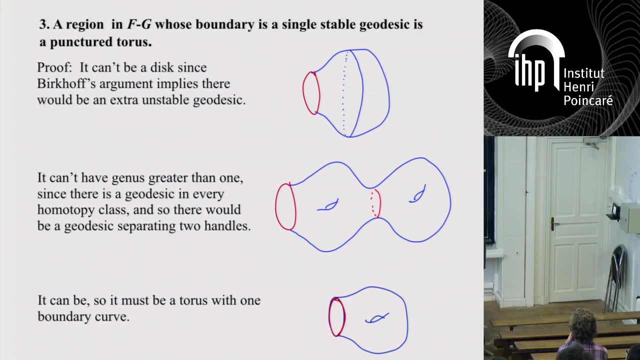 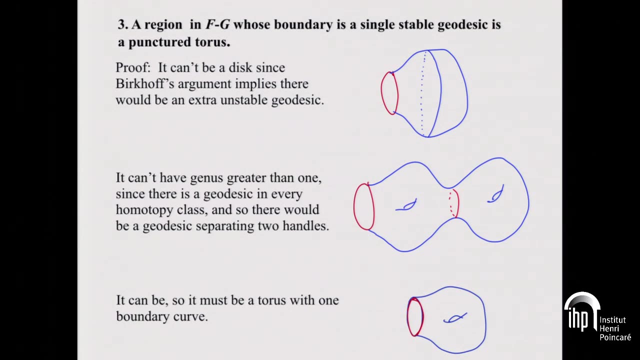 Or it could bound the surface with genus one. Now, if it had genus, if it bound to something of genus more than one, then we could separate those two handles by a curve and take the shortest curve in that homotopy class, and that would give us a separating geodesic, which we assume that this region had no more. this 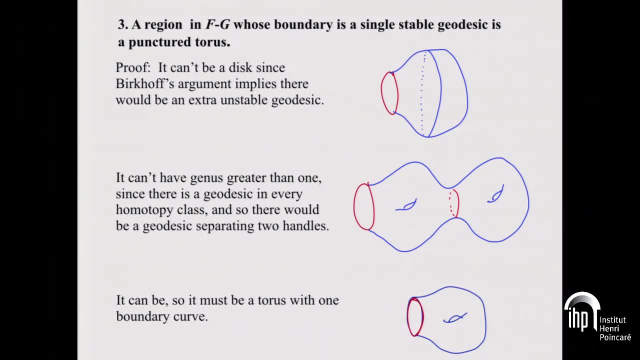 is a region which has one of the original family and its boundary and no more separating geodesics exist None inside it. So we can't have genus more than one or we wouldn't have had a maximal family. So the only possibility is that it must bound a-. 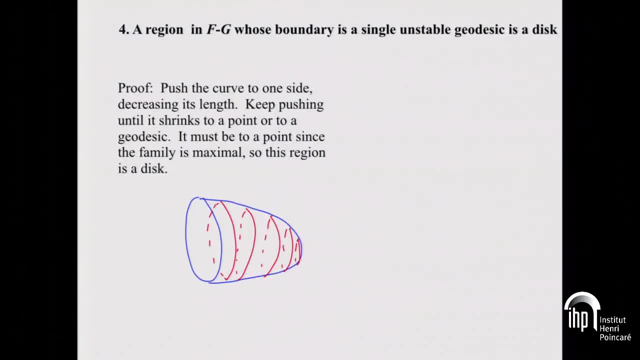 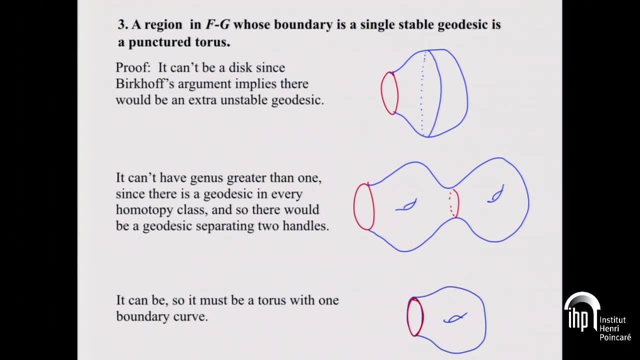 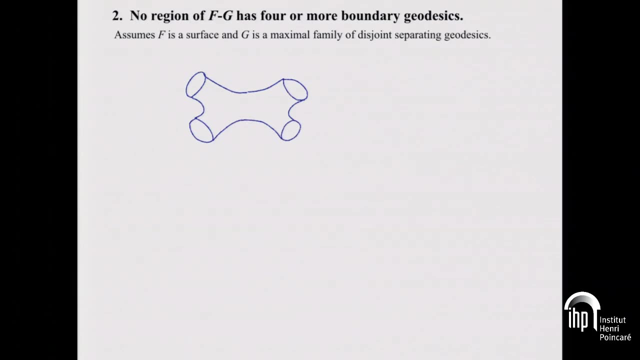 Question about that last case. Yes, There's a homotopy class of curves going through the pole. Yes, Going around the right, That's right. Where did that go Right? So- Good question. So if you look back at so, I was hopefully careful to state this and said G is a maximal. 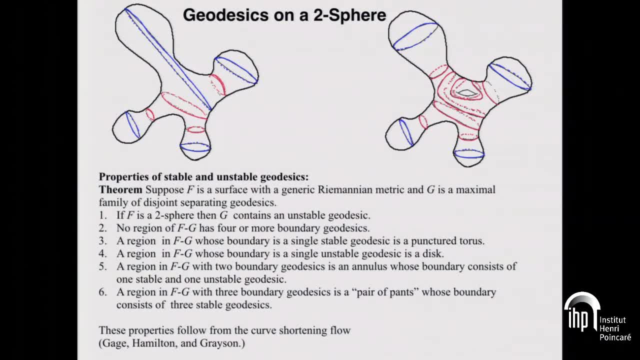 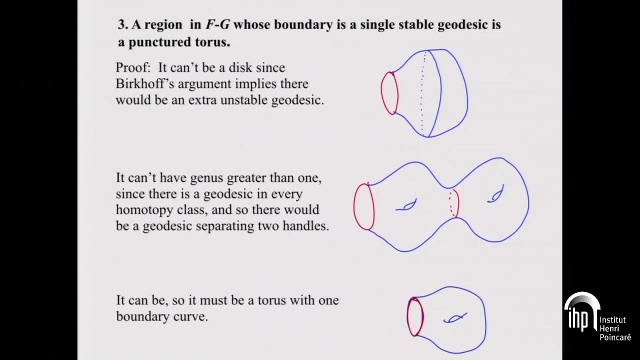 family Right. So G is a maximal family of disjoint. separating geodesics. So I'm only looking at separating geodesics. The geodesic that goes through the hole is non-separating. There are many more geodesics on this torus right. 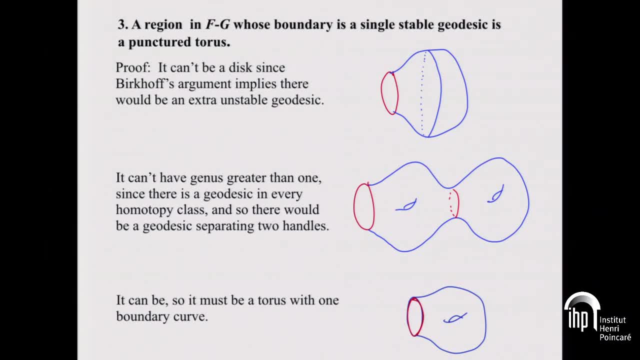 There's one that runs around like this or like that or many others, but each one of them is non-separating. So I have to throw that in for the surface, For the three manifold. when we're looking for three spheres, we can, as a first step, 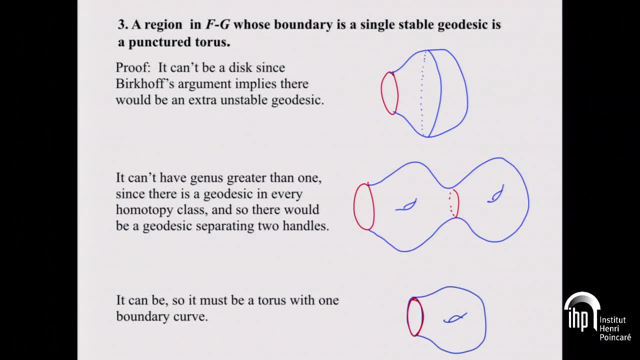 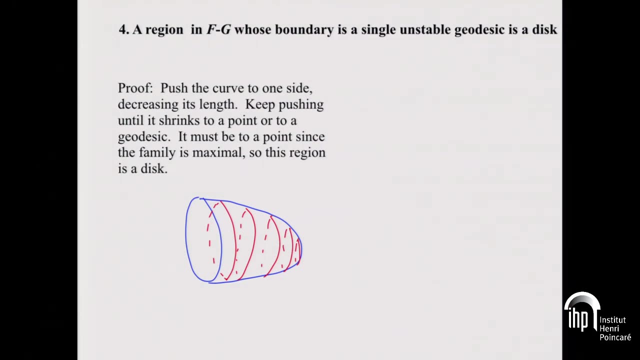 assume that the manifold is a homology three sphere, that everything is separating, because that's very easy to check computationally. But for surfaces that would eliminate everything unless- So I'm adding this condition of separating to the curves. So what about a region which has an unstable geodesic, a single unstable geodesic? 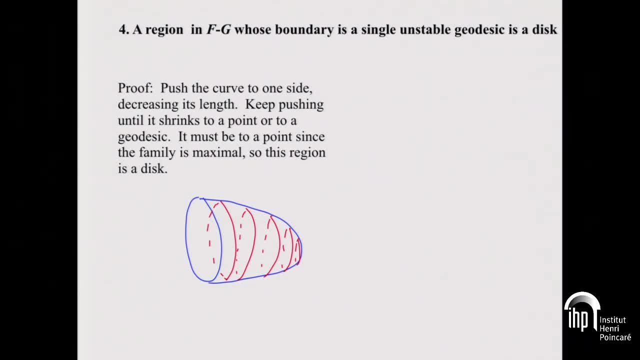 So this one- Because it's unstable. we can push it off. We can push the boundary off a little bit and decrease the area. That's what being unstable means. But now we can keep on shrinking that curve until what happens? Either it shrinks to a point, in which case we have a disk, or it shrinks to some geodesic. 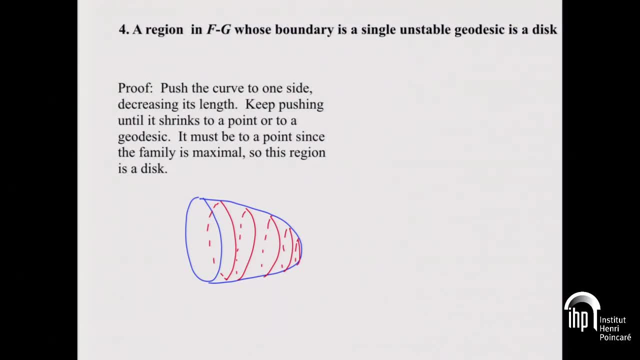 where it gets stuck, And in that case we again don't have a maximal family. So the only thing that can happen is it bounds a disk if it's unstable. So that was case four. What about a region with two boundary components? 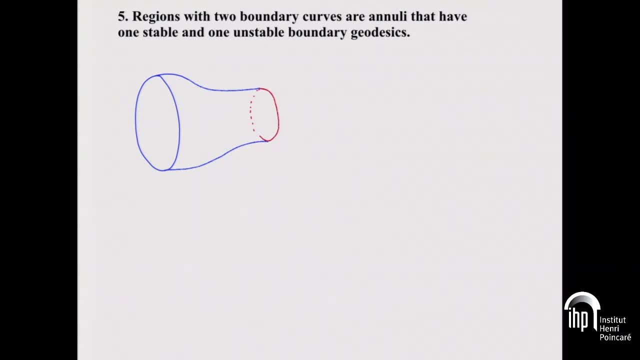 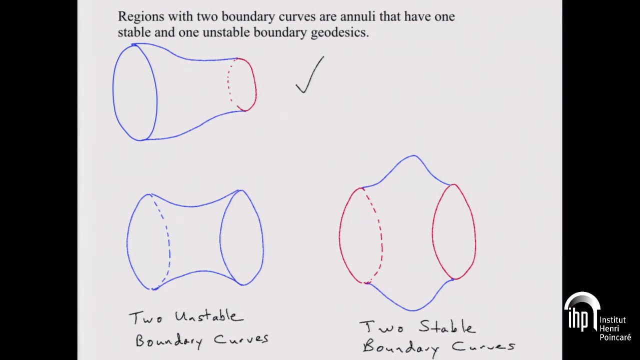 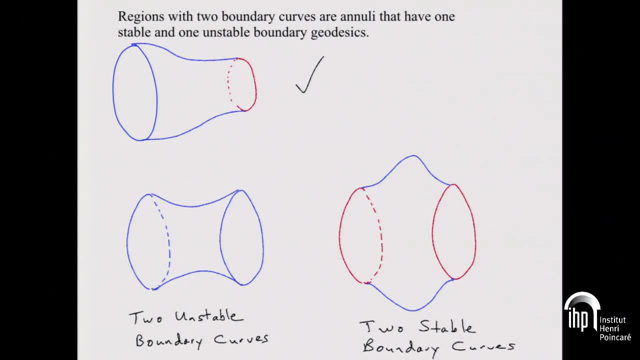 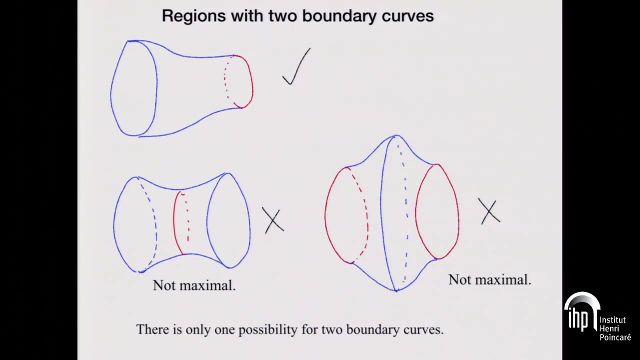 What would happen? What would happen, Oh, If it had two boundary components. that was not of this type. Maybe it has two stable or two unstable boundary components. So if it's got two stable boundary components, then when we uh it. 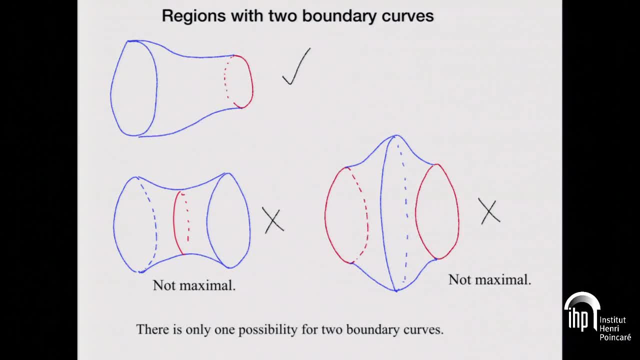 It should be. excuse me, so this left one. if it has two unstable boundary components, then we can push each one of them in and each one of them will converge to some stable curve which does not lie on the boundary. Maybe it's the same one if they co-bound an annulus, or maybe it's. 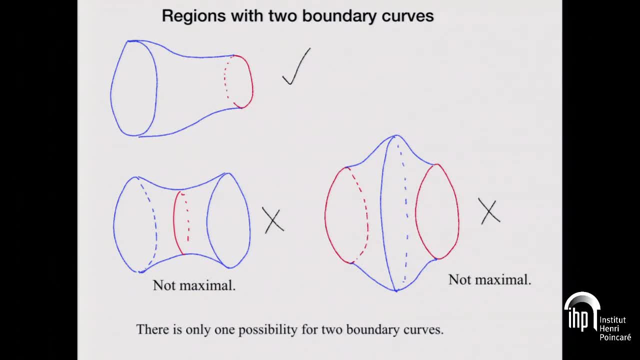 a different one, but in either case our family was not maximal. And similarly you can rule out the other case. You push in and if those two boundary curves are homotopic, if they co-bound an annulus, then you get an unstable one separating geodesics inside. 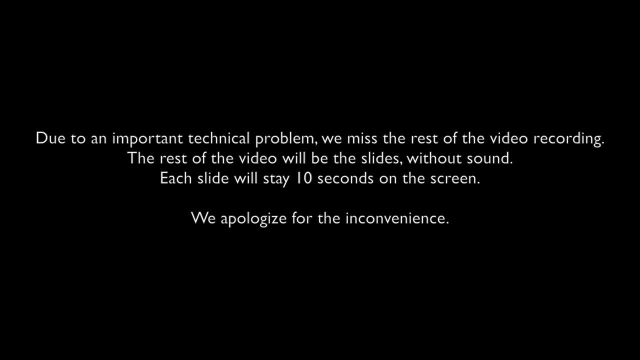 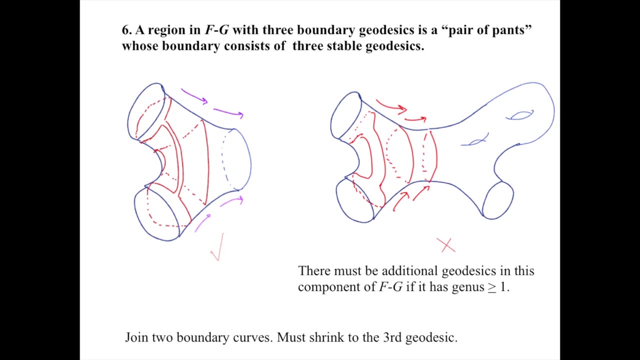 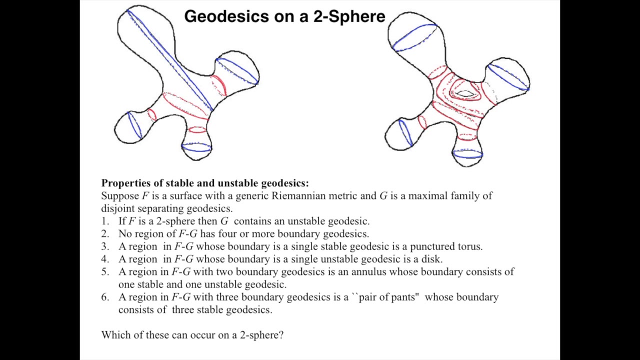 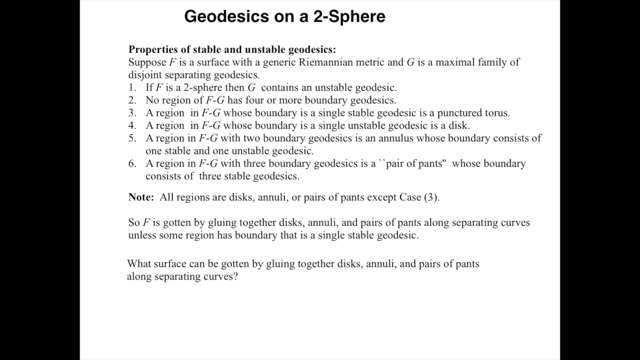 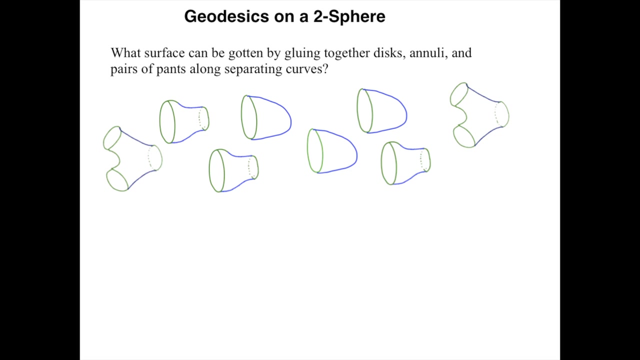 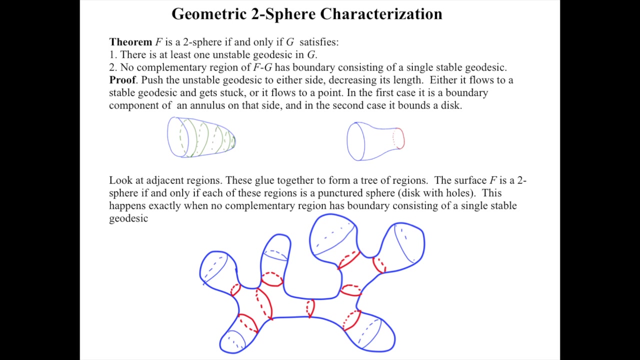 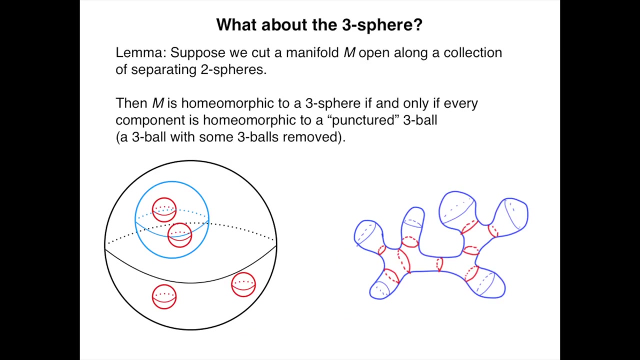 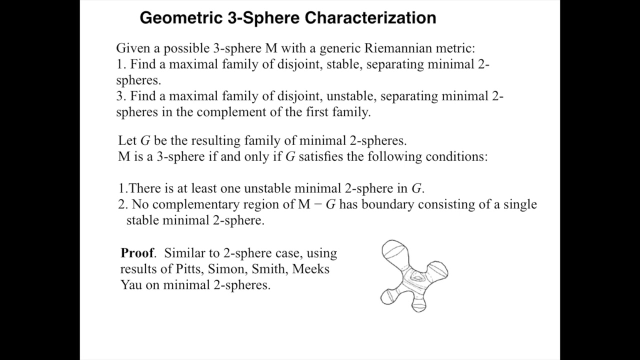 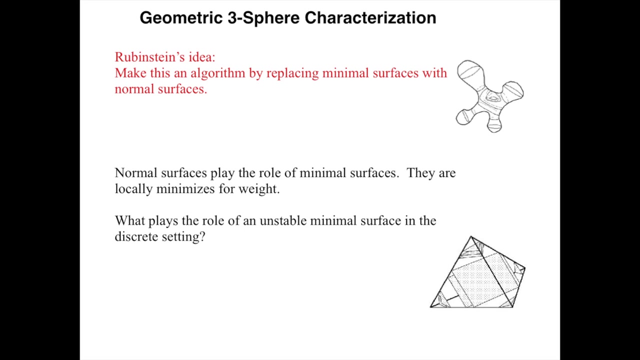 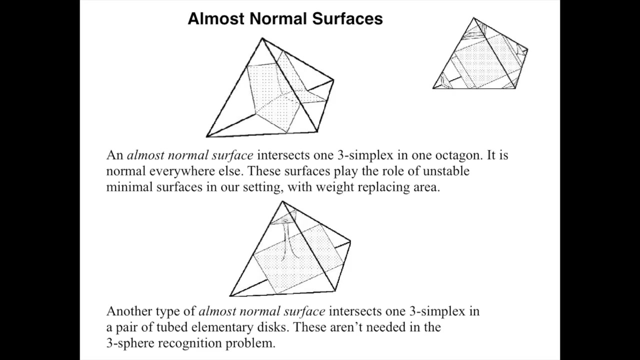 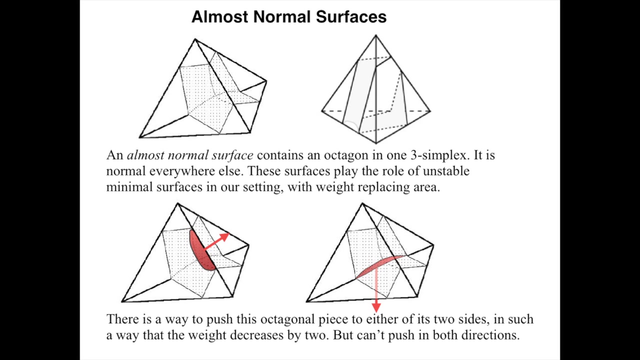 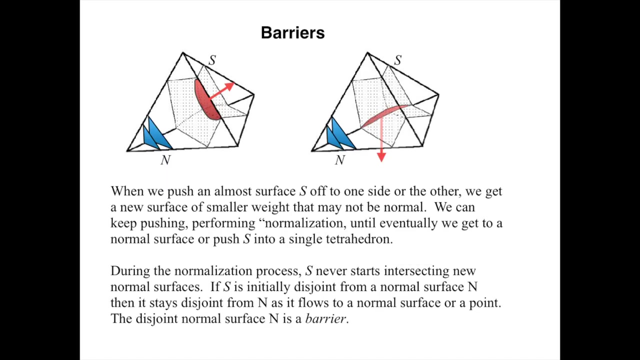 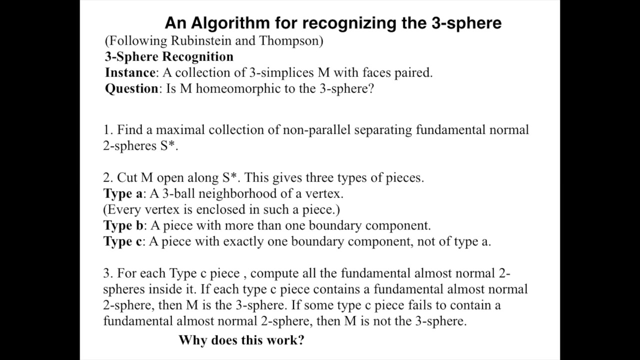 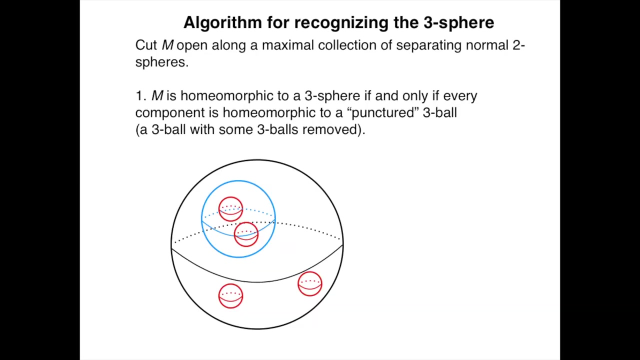 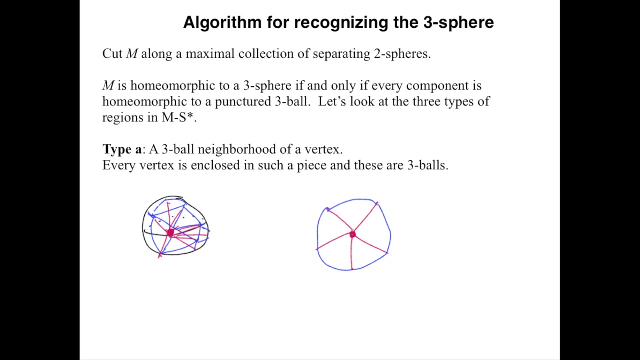 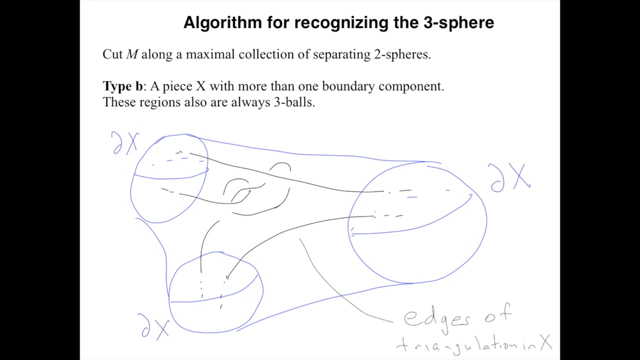 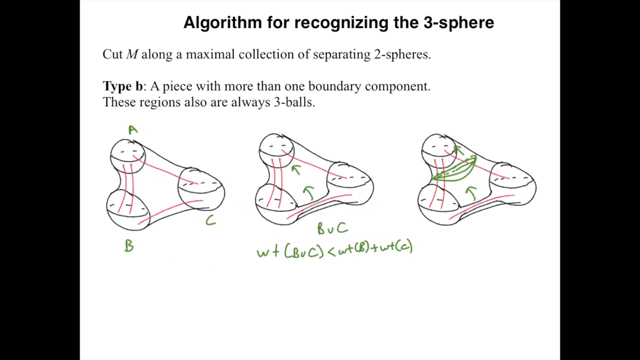 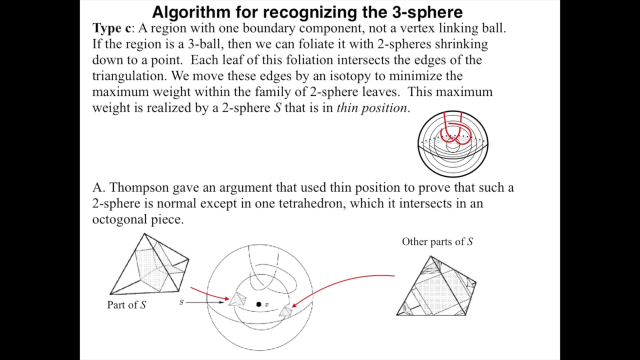 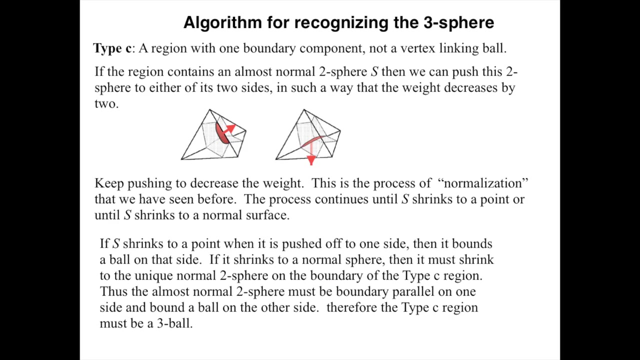 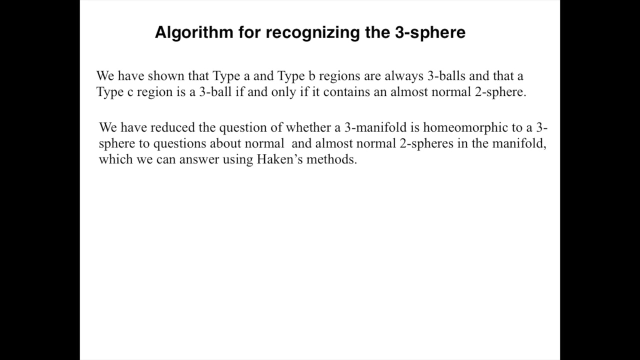 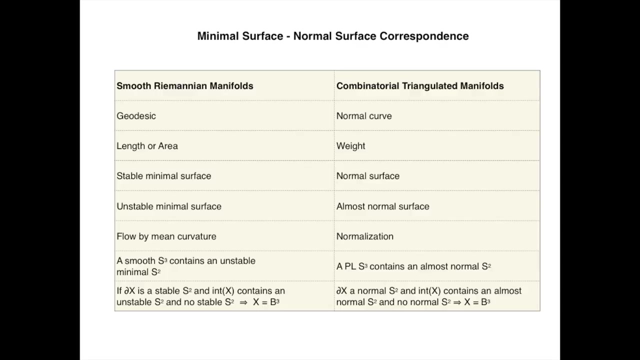 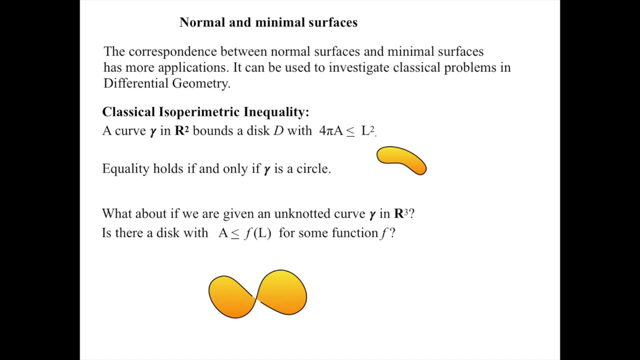 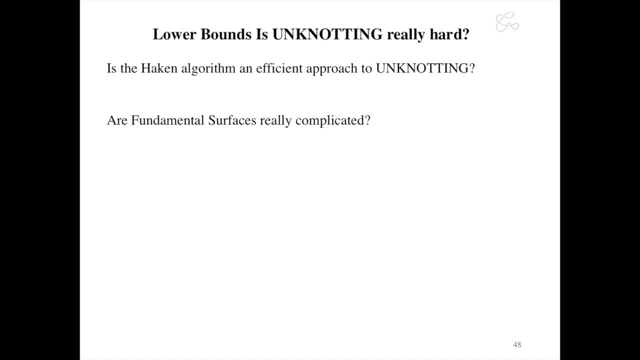 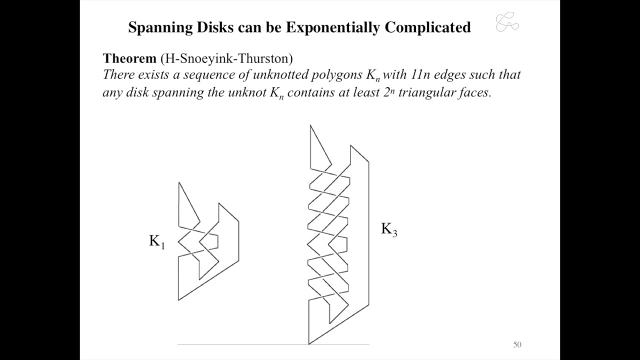 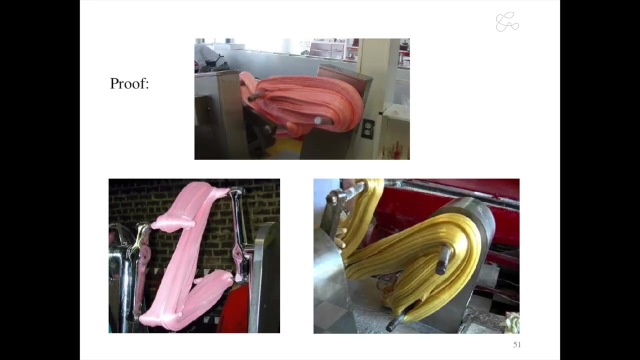 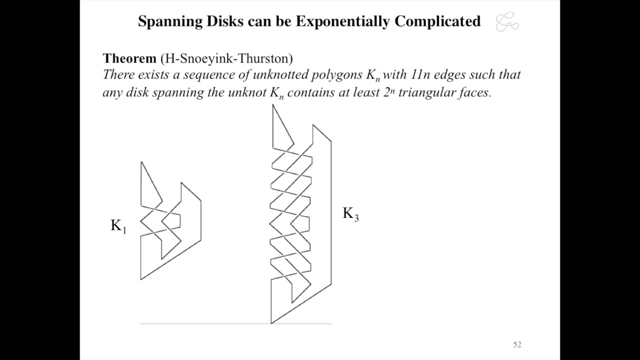 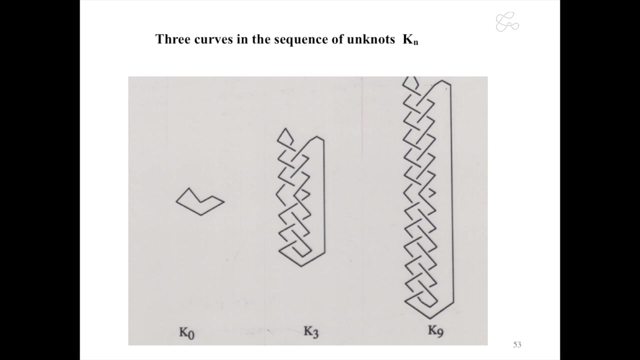 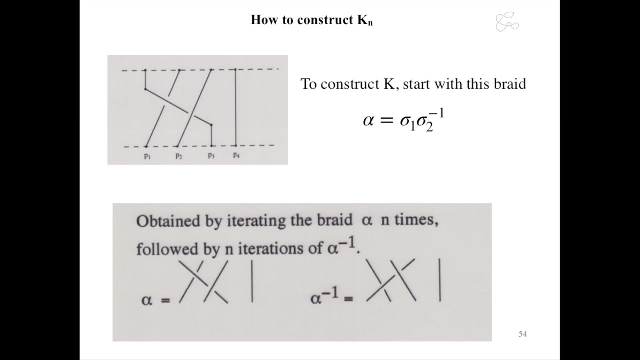 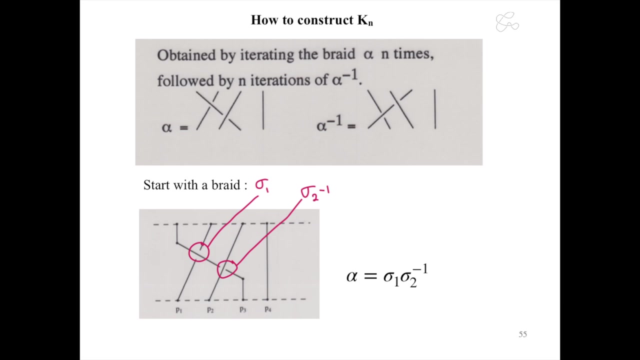 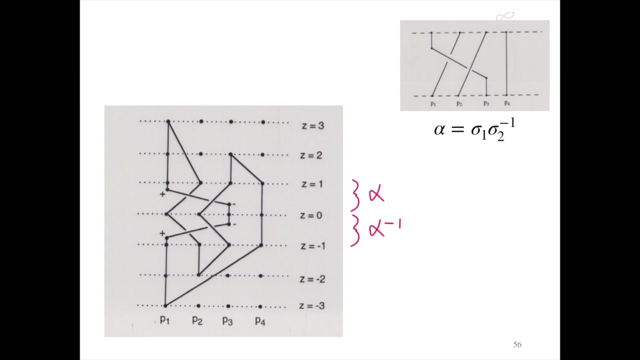 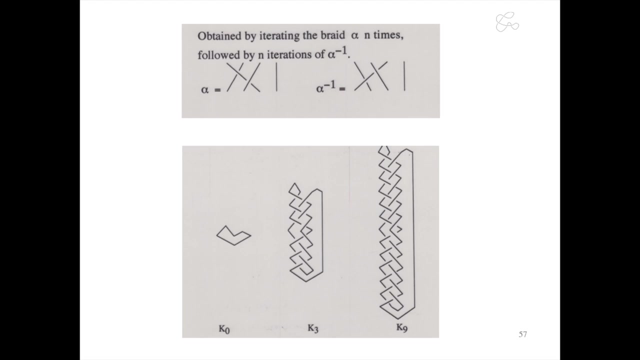 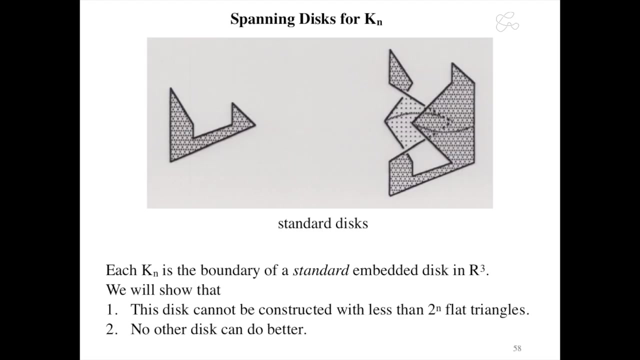 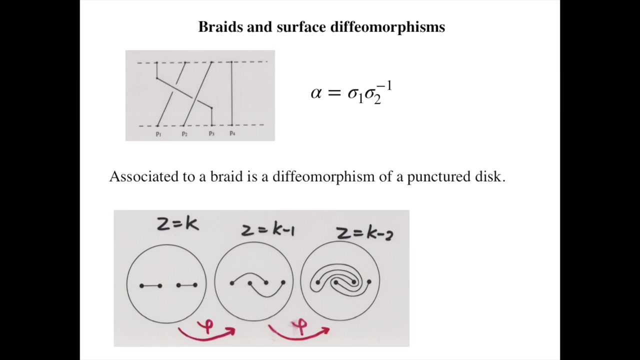 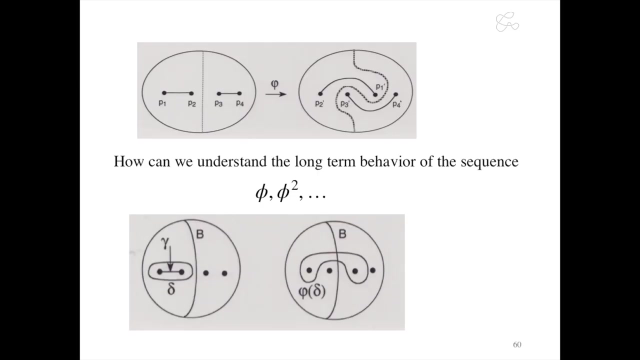 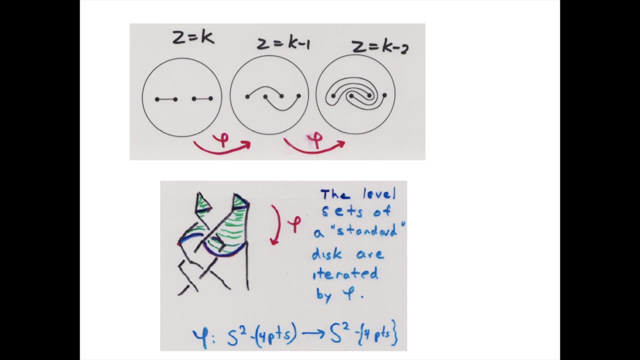 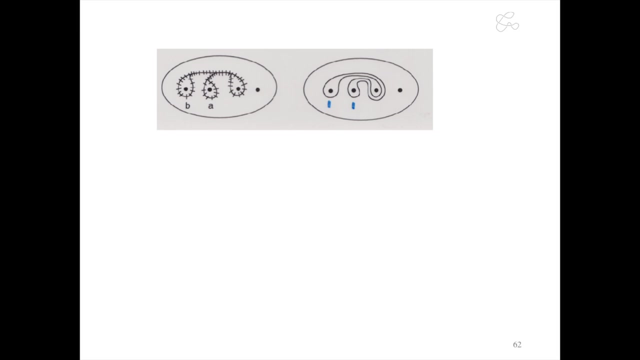 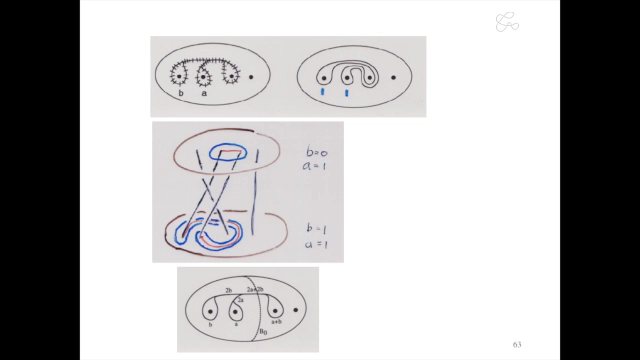 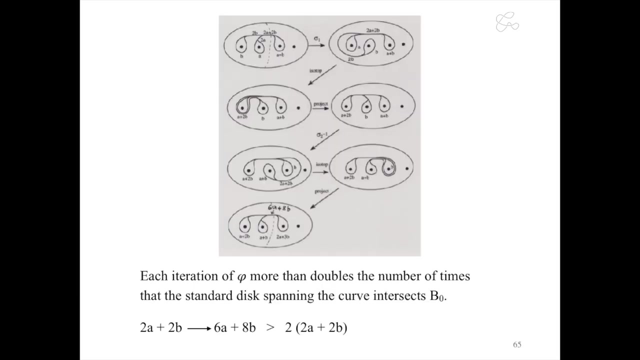 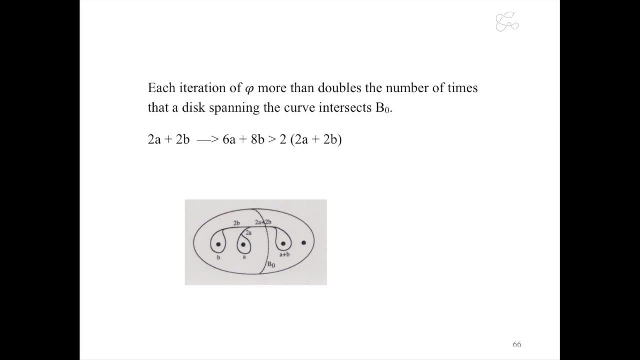 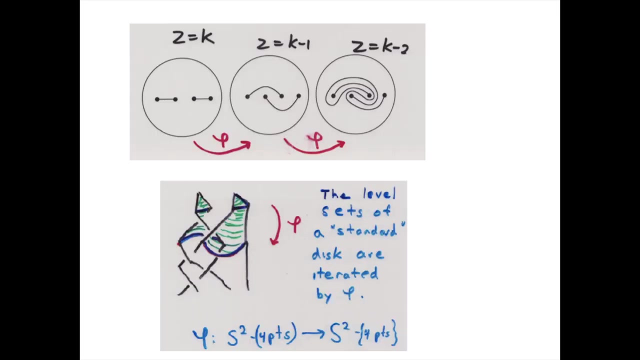 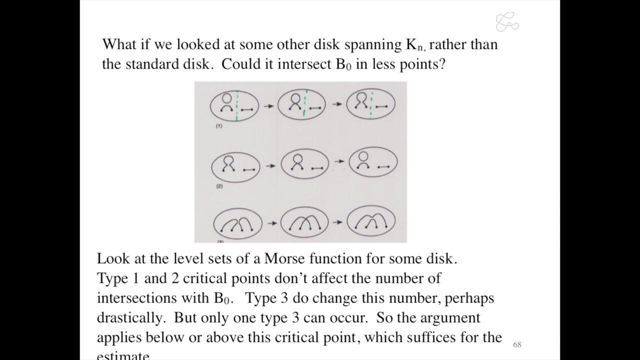 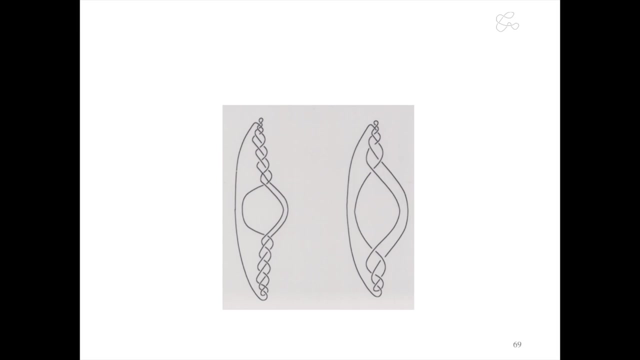 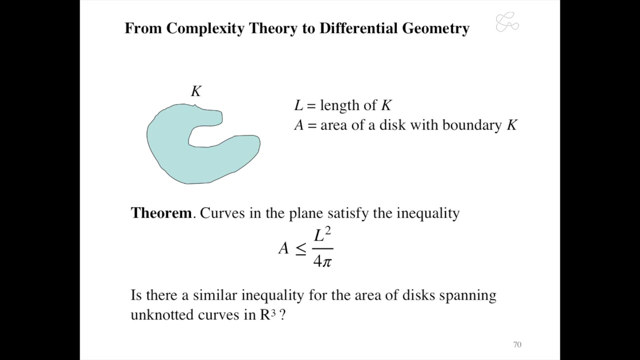 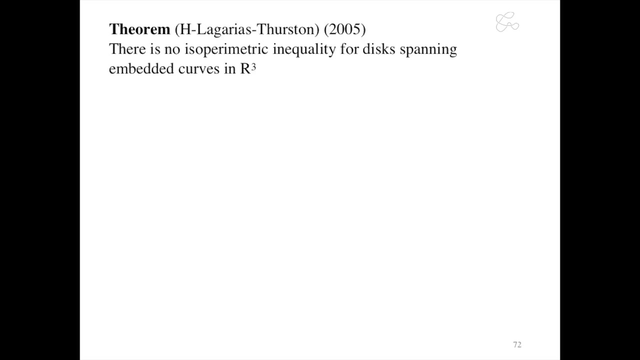